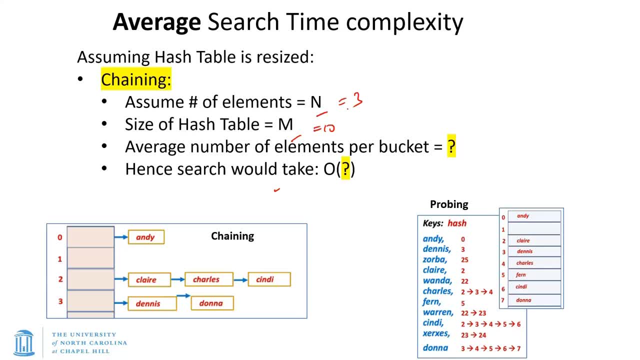 you have, uh, three elements in it. so what is the average size or average occupancy for every location inside the hash table? from the straightforward, yeah, yeah, exactly. so it's simply n upon m. all right. so n upon m uh is simply the number of elements per index location or per bucket, as you might refer to that. 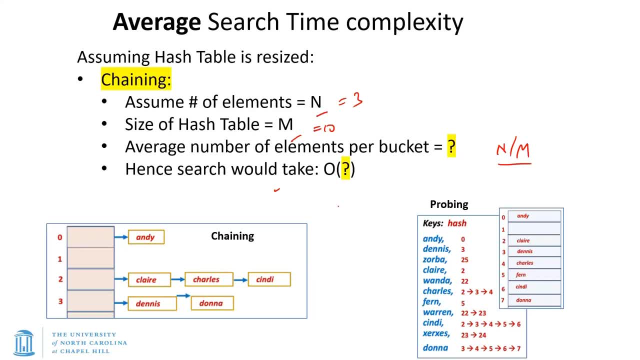 all right, um, now the question. the next question is: how long would a search take? so now, remember, we're doing hashing. so how do we do the hashing? we initially calculate the hash function. that takes constant amount of time. all right, so if you might say, the order of complexity is initially one. 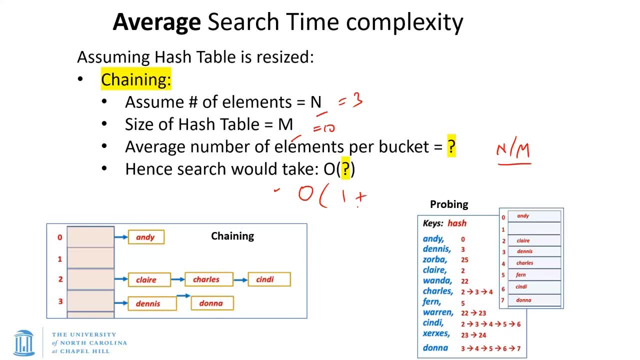 because we're computing the hashing function and then we get to that particular location and we're doing the chaining analysis. so now we have to see how far down the chain- the linked list- we have to go. and how far would that be? how far down the chain do we have to go on average? 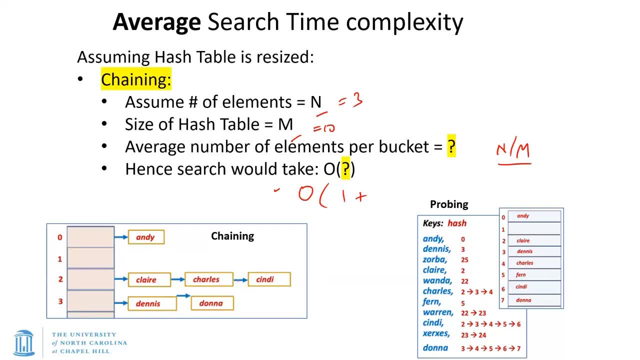 yeah, right, so the worst case is bigger of n. what about the average case? um, think about what we just discussed. yeah, o of one. but what if i'm not restricting n? i'm saying n could be 100 and m could be 10.. you're saying the average size of the linked list is n upon m. 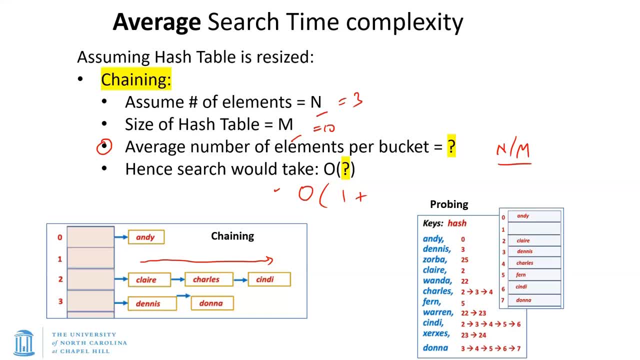 so what is the average number of steps that you have to take? yeah, n divided by n, right? so we're saying that, you know, let's say that the average size in this case is 1.5. okay, so you basically go n upon m steps on average- not the worst case, but on average. 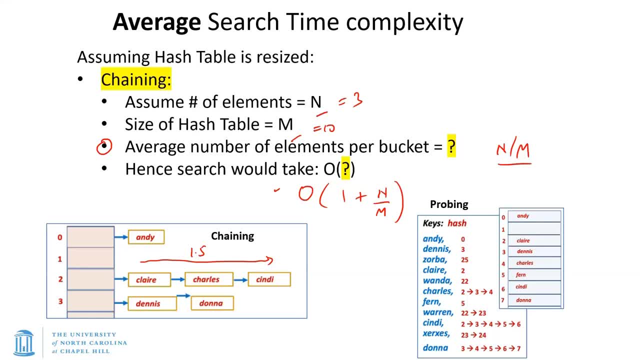 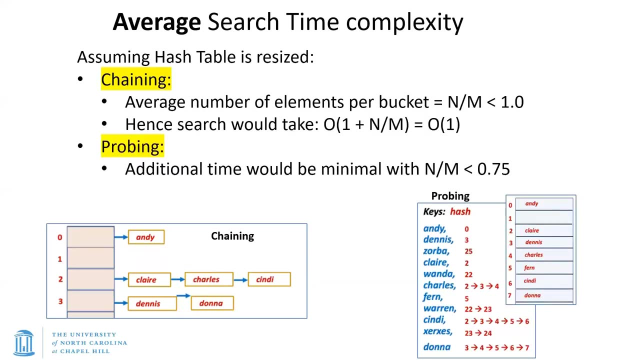 does that make sense? so initially do a computation, computation the hash function, and then we get to that particular location. you go down that series of linked lists on average n upon m steps. okay, but let's say that n upon m is now fixed. okay, we are now resizing. so we sort of 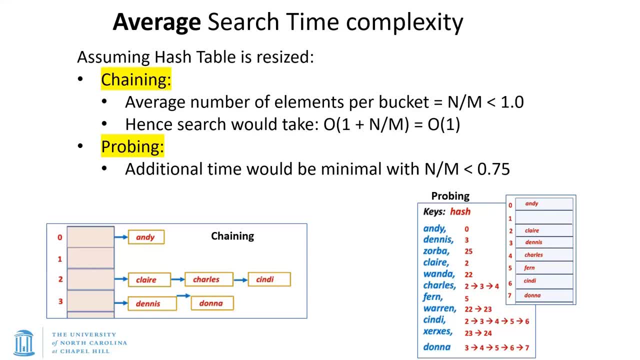 guaranteeing that as the hash table becomes congested for the chaining case, let's say we are taking the threshold to be one. as soon as you hit n upon m is equal to one. you resize. now we're doing a search complexity, so we're not looking. 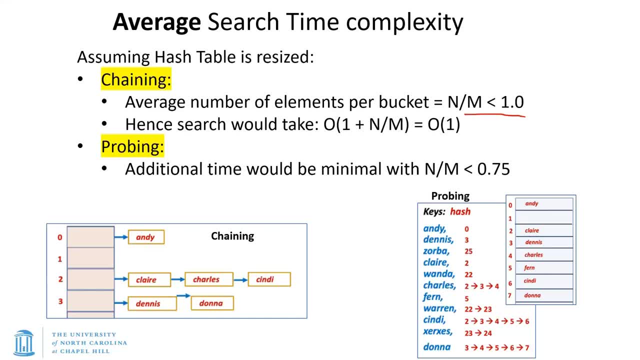 at the time to do the actual resizing. assume that that is already done. so if n upon m is now guaranteed to be at most one, then the complexity of a search would simply be one plus n upon m. now n upon m is guaranteed to be less than one, less than equal to one. let's 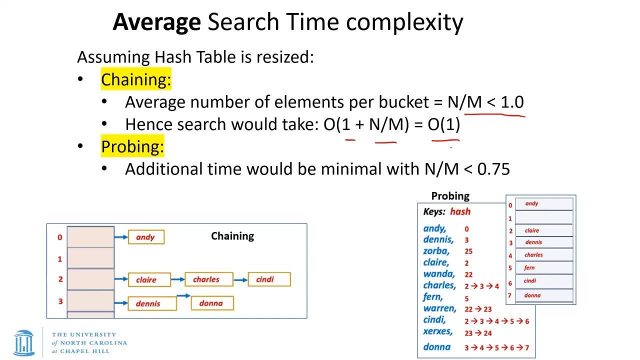 say so. in any case, that comes out to be order of one complexity on average. okay, yes, yes, if you are resizing. so as long as you're doing resizing, we, the internal function, will ensure that as soon as you hit that threshold, you're going to resize. okay, so, um, so, the complexity for chaining comes out to be bigger of one. 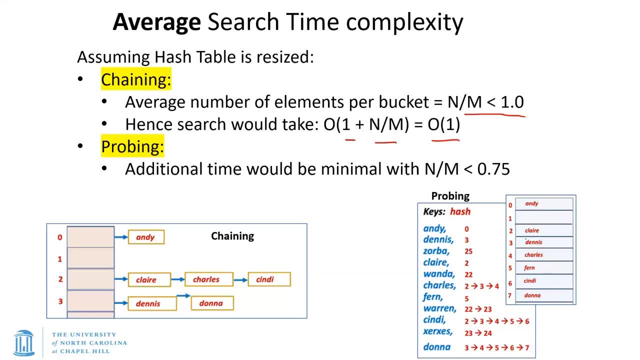 um for probing. uh, we are saying that n upon m is even smaller, all right, so remember, we said that the thresholds for uh probing would be slightly smaller because it has a very hard it's. it's a closed, uh, it's a closed scenario, okay. so, in any case, 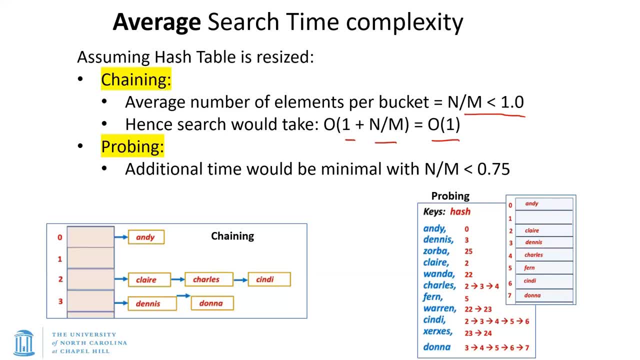 even if it was one or less than one, or even if it was two, it doesn't really matter. as long as n upon n has a bound as a constant bound, then the search would simply take order one. okay, so that comes out to be the complexity for doing a search. 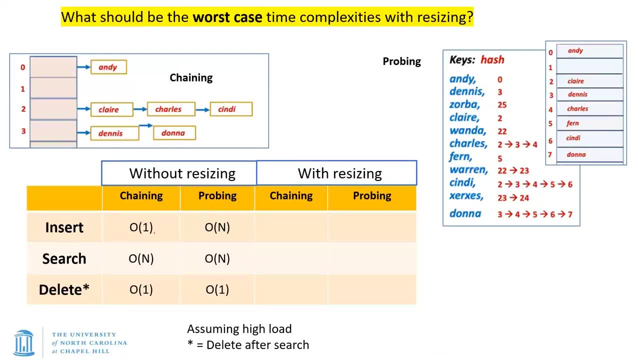 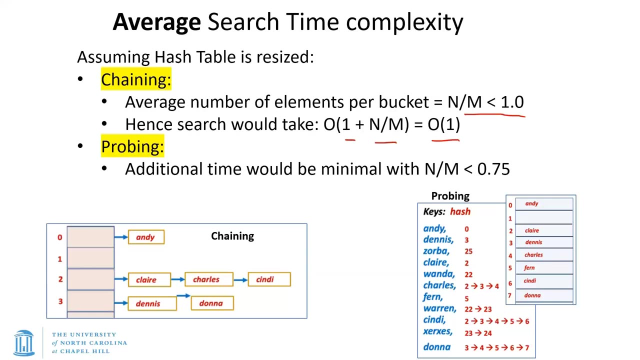 okay. so, um, in chaining, we have uh order, one order of n, to do a search. but now let's take think about uh, insertion. okay, so, let's think about insertion. i showed you a glimpse of the next slide but, um, assuming you didn't see that, let's think about insertion. so, chaining versus probing, okay. 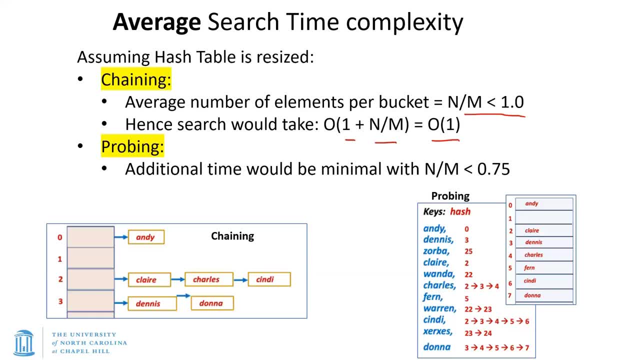 with resizing, things are becoming a little bit more complex. all right, we're not just doing ushing, but now we're also doing resizing. okay, so if you're doing an insertion, what would be the worst case? complexity? so let's say you do an insertion in the chaining case, we say, well, uh, let's say, um, we insert at. 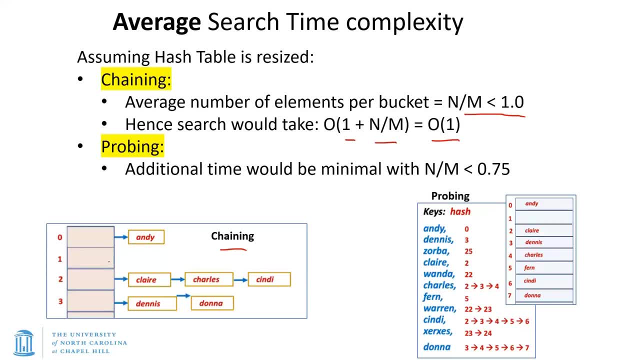 this particular location. so let's say we and we're adding bob over here, all right, and that should take a constant amount of time to do the insert. but at work, but is bobby's not bad? but is bobby's not bad after that? oh, all right, that is still in cloud. that insertion would take constant time, okay, yeah. 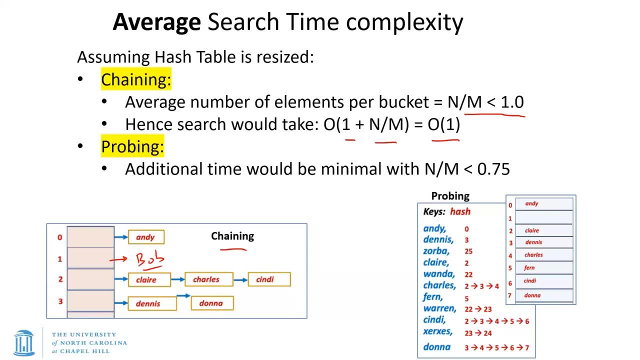 yeah, exactly, so you may have to resize, right. so in the search we didn't have to do a resize. but when you're doing an insertion it's an array list, presumably underneath, and so you may have to resize the hash table, and you know that implies that you have to not only copy all. you have to first of all create. 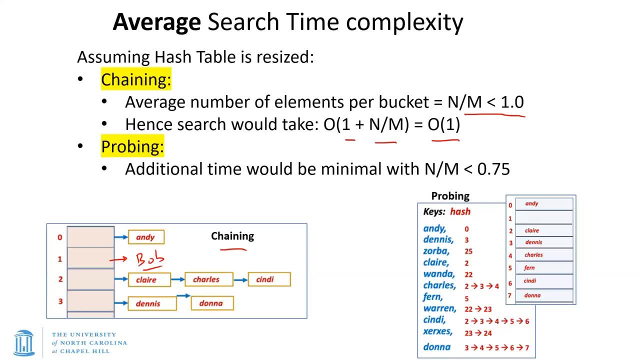 a new array list. you not only have to copy them, but you for each copying you have to actually type in the hash function. all right, and so that would take big o of n. okay, so an insertion would be a big o of n, simply because underneath this there is an array list that has to be resized. so 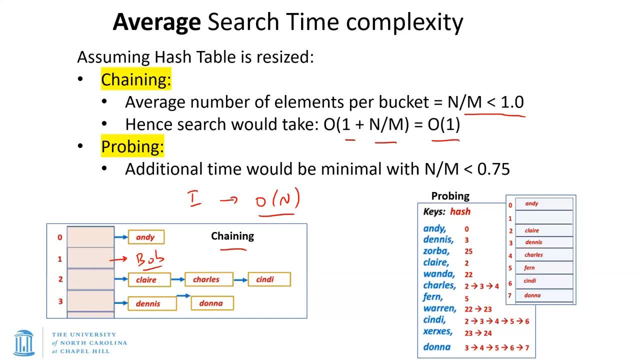 now we're talking about resizing. the worst case is going to be the go home. okay, now, in this scenario i said that this is the average scenario, but, um, you can also say that if you have a good hash function, then you can assume with a very high 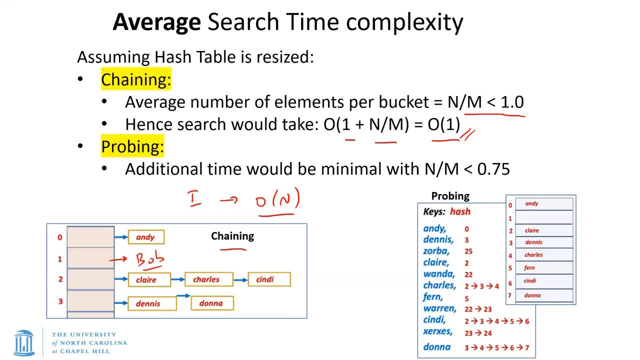 probability that you have a good hash function, then you can assume with a very high probability that it's going to result in a very well distributed um insertion. okay, so if you, for example, if you're using double hashing, you've already seen that. so if you're using a good 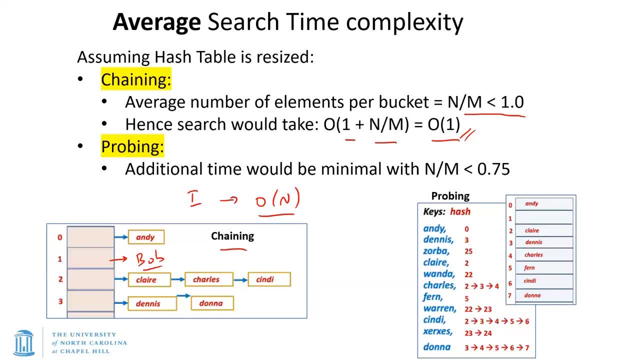 hashing function, which presumably we always will- then that's going to result in a very well distributed insertions, so you won't have the scenario where all of the elements are in one long linked list. okay, so this can be thought of as the worst case as well. okay, so if you're doing a good hashing function, 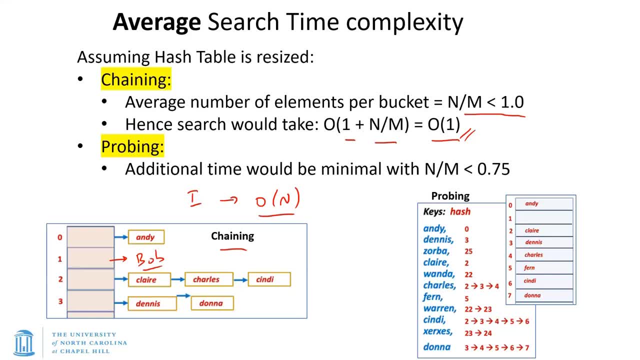 then, uh, even in the search scenario, it's going to be big off one. however, the insertion is going to be big off end simply because you have to resize. okay, now let's think about um insertions for probing. if you're doing an insertion in the probing scenario, you're already assuming that we're 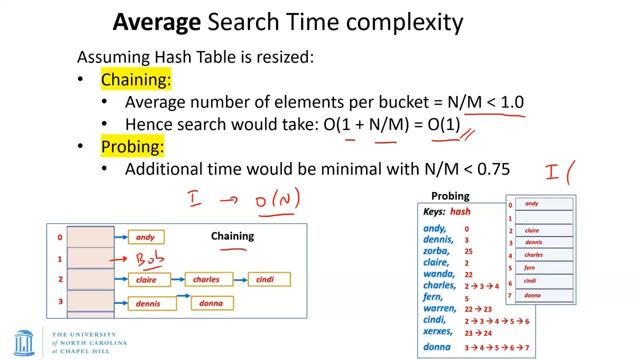 going to be ficcizing square from the one we had in theka and route to what might be little bit less than one. how big is our hashing function? things like we've seen before and we're going to. we're going to divide in half by point one, so that's what you can suppose. 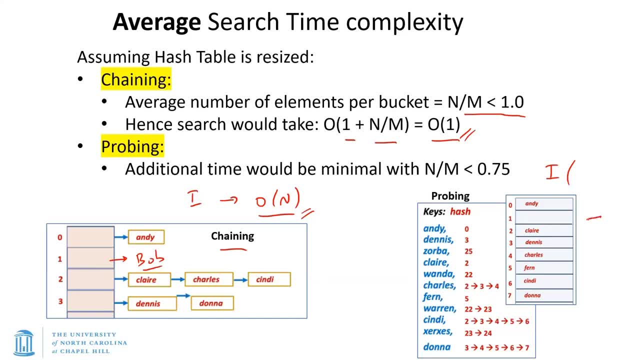 you can, whose hashing function is gonna be? and you say, well, let's say you're trying to insert some other name starting at C, right, So you're inserting Cindy- well, Cindy is already there, but let's say we're inserting some name- CX- okay, 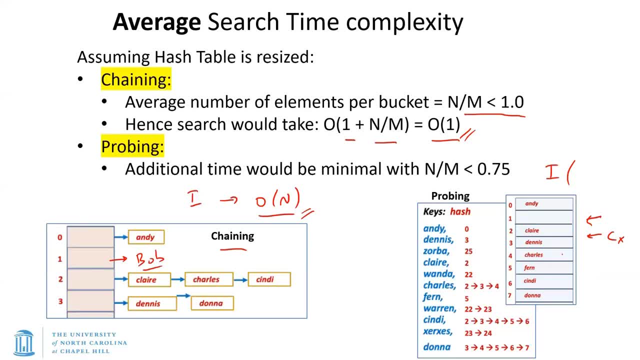 So now we already guaranteeing that n upon m is going to be relatively small as compared to the upper limit of one. okay, So it could be 0.75,, it could be 0.5, it could be 0.6.. 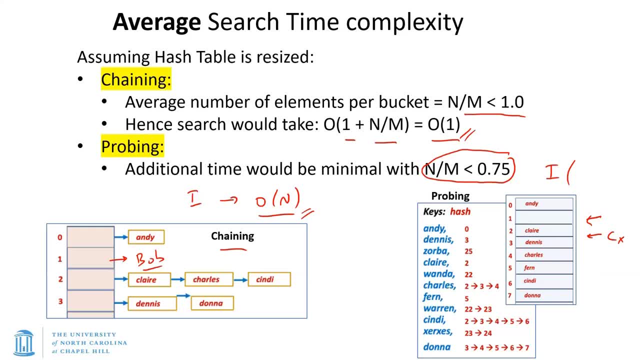 Now, without proving this, I'm going to tell you that the average time to actually do an insertion is going to be bounded. Why is that? Because if it's a good hashing function, there will generally be spots not very far away from where you're trying to insert. 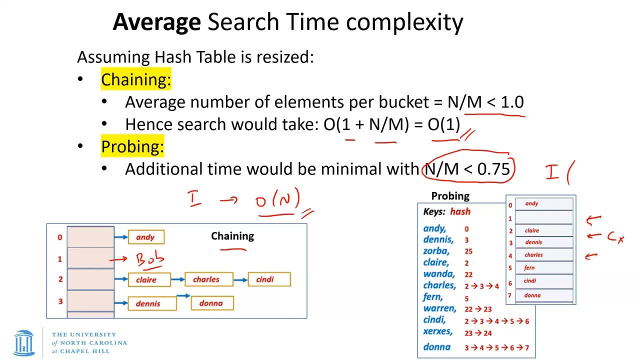 where there will be an empty spot. okay, So you won't have to go all the way around the array. okay, You'll probably go one, two, three, four, five steps, but it's not going to be very big. 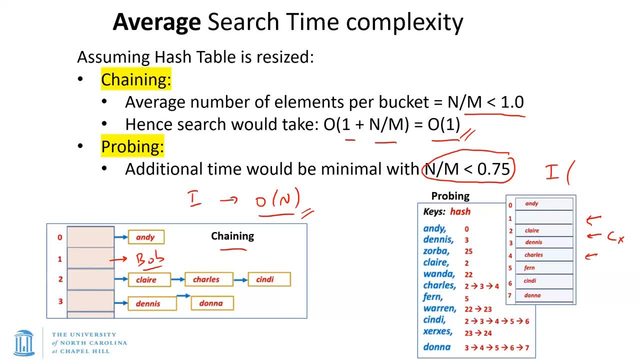 Simply because you're assuming that it's a good hash function, okay, And you are ensuring that n upon m, that means that maximum 75% of the slots will be used up, 25% will be available. So those 25% of the empty spots in the hash table. 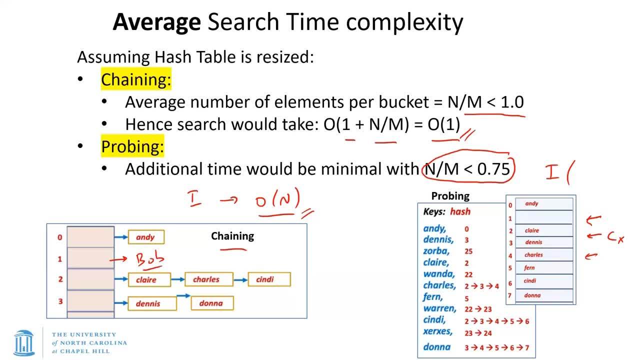 are going to be spread out fairly uniformly, So you generally shouldn't have to go too far to be able to do an insertion. okay, So insertions are fine in terms of actually finding the, but then what is the other problem? What is the other problem? 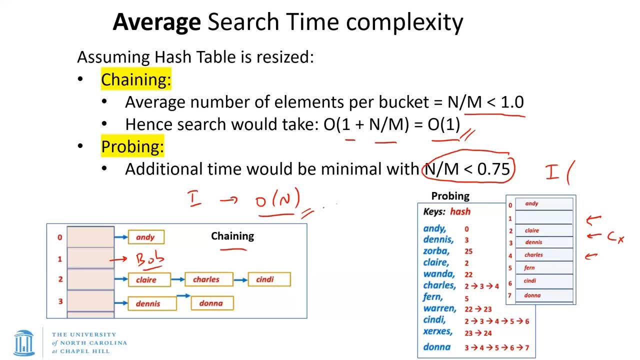 It is just like in this particular case that underlying it is a hash table And if that particular element results in the threshold being crossed, and all of a sudden you've inserted n, such that n upon m is now bigger than 0.75,. 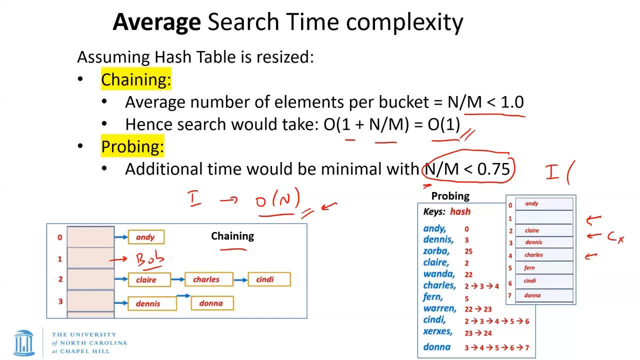 and all of a sudden you're going to have to resize And that's going to take forever, okay, So insertion wherever you have hash tables, sorry, wherever you have an array list being used, regardless of which data structure you have. 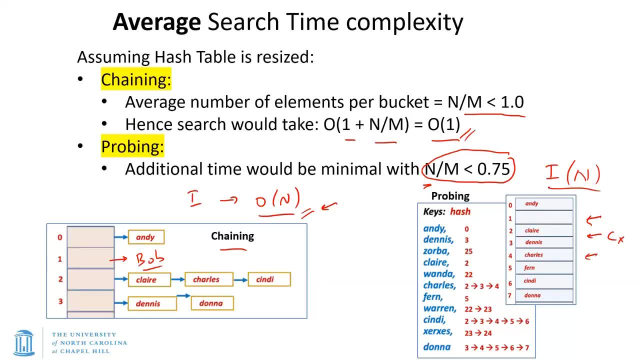 it's always: the worst case is always going to be bigger than Okay, worst case. So insertions in both cases are going to be bigger than What about deletions? What about delete star? So let's say you've actually found what you're looking for. 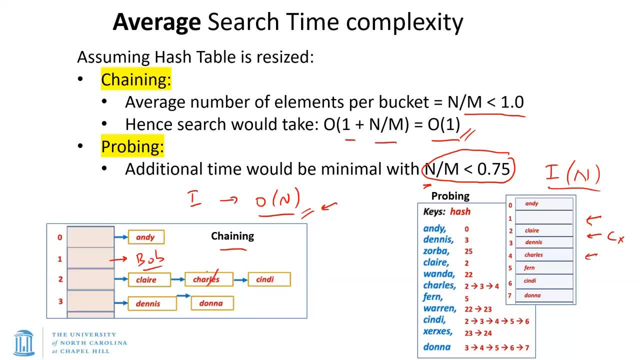 so you found Charles and you kind of delete Charles along with that day. Yeah, But if you delete Charles, say that again, Yeah. so remember you have to resize both at an upper threshold and there's also a lower threshold. 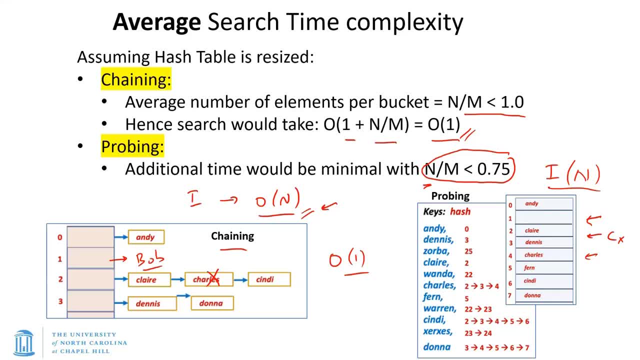 So the low threshold is crossed and now, because of that deletion, we have to resize and make it smaller. so that's going to result in an order of n. So even the delete star is going to be order of n. for chaining, What about for probing? 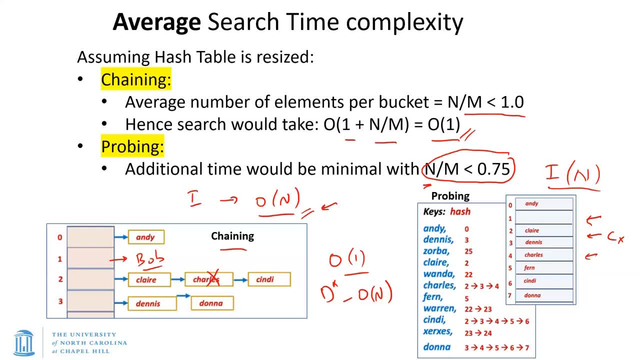 Yeah, Exactly So, it's the same thing. So as soon as you've found what you're looking for, you delete it, and n upon n goes below that low threshold, so you have to resize. So both delete star. so here we have, these results. 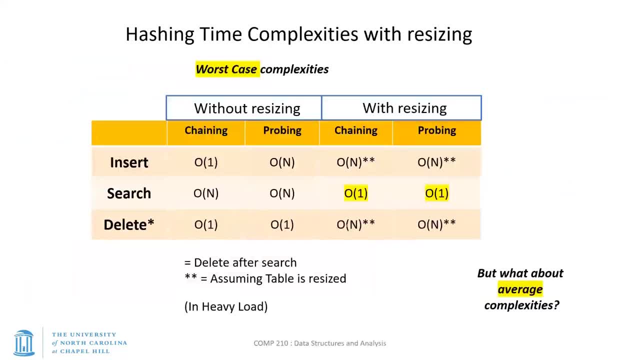 Now we're talking about width resizing. so we've just seen the following scenarios. We said that if you are inserting, then insert for both the cases is going to be bigger than n. If you're doing a search And you have a good hash function, then even as I said in the example of probing, you won't have to go too far, okay, 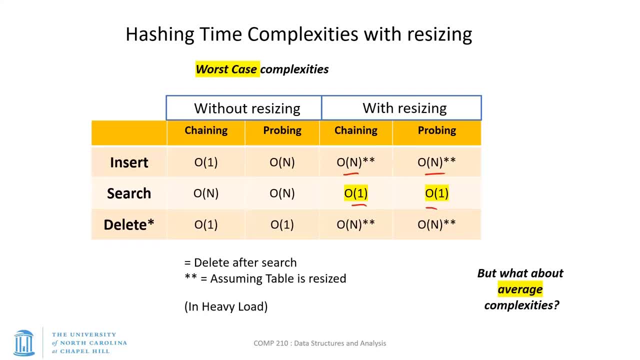 So you won't have to go all the way around simply because you've got a well-distributed hash function. You're ensuring that maximum of, let's say, 75% of the slots are used. So you may have to go a few indices down, but you won't have to go all the way around. 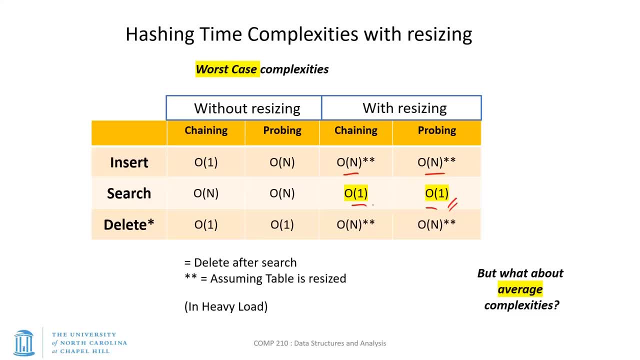 So you can say that. you can see that in both of these cases, You're going to be seeing bigger one complexity Delete, however, simply because it's going to be resized. In all of these scenarios, you're seeing a resizing, so you have a problem, okay. 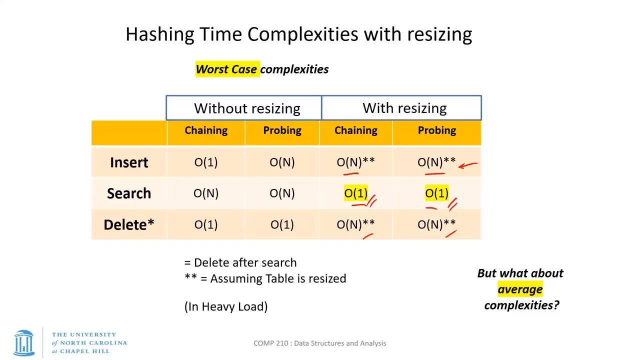 So now it doesn't look very good. I mean, we thought hashing was really good, but it seems like it's not so good right? Simply because the only thing it's good for is search, but if you're doing insertion or deletion, 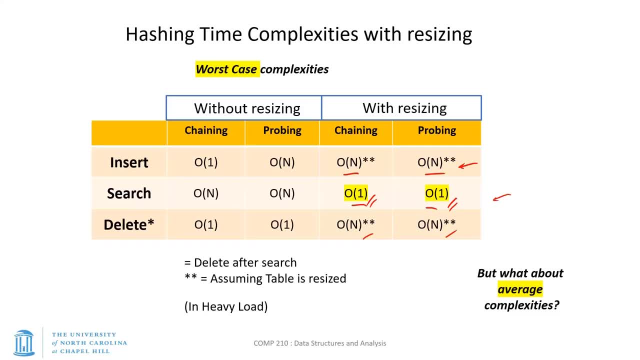 you have a problem And we already saw that it's no good if you're trying to do- you know, trying to do an enqueue or dequeue for a priority queue. So we discovered that. So what is it good for? Well, remember, amortization, okay. 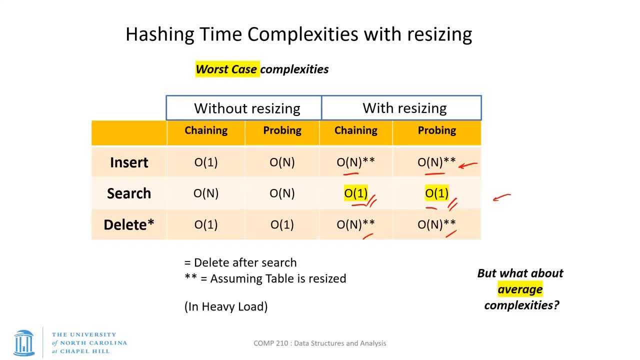 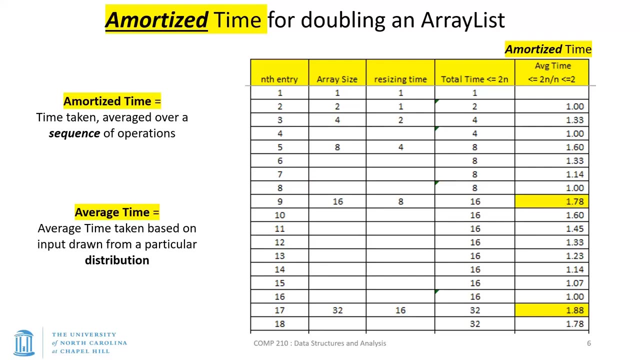 So now you know it's not always good to look at the worst case, as we discussed earlier. Generally, it's a good idea to look at averages, And amortization has already shown us how to do this. We discussed, So we know that if you're doing, if you're looking at the amortized, amortized average, 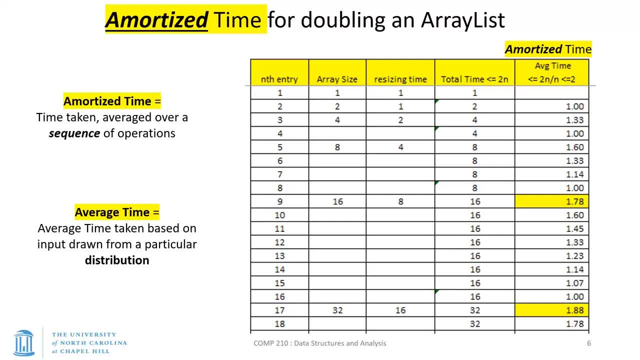 if you're working with an array list and you have to resize, then the order of complexity is order of one, okay. And even if you're doing a resize and you're making it smaller that without actually going through all the entire process, 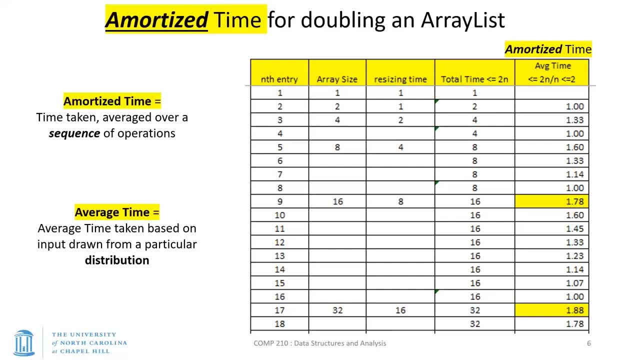 you can take my word, for it is also going to be bigger of one, okay, So? So, resizing amortized averages are order of one, and we've already seen that earlier. So now, if you include that and you say, well, what about the averages and the averages? 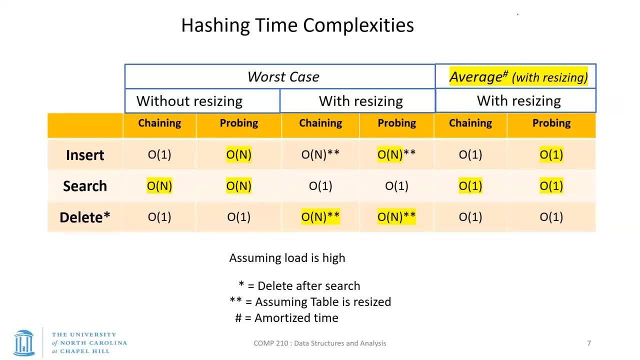 We are going to be assuming that we're talking about amortized averages in this course. So in that case, what happens? Resizing is not a problem. okay, With resizing is not a problem. then, all of a sudden, all of these worst case scenarios. 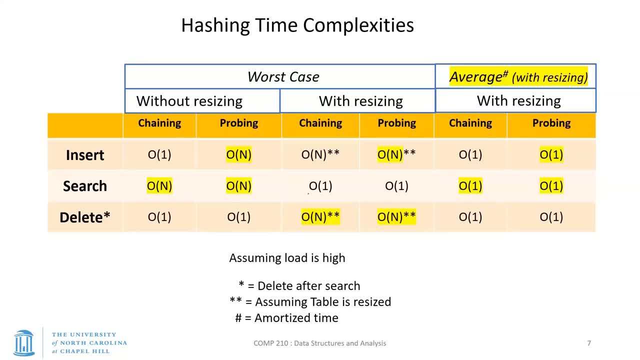 actually start looking pretty good, okay. So worst case is up here and this is the average scenario. And we're saying that here you have these four scenarios where, because of resizing, you have a problem. but if now you look at the average based on amortization, 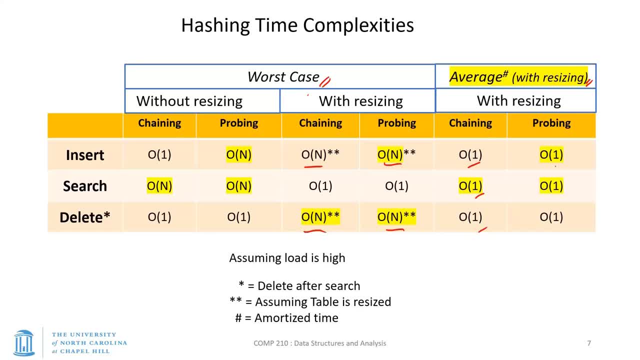 then you simply have a tremendously positive result. So this is sort of an Okay, Important point, the important point. if there's one point in this course where you know you I should open, you would say, wow, all right, so this is the point. 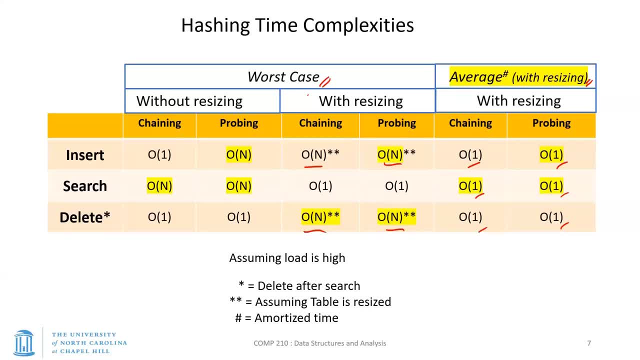 So now you've got a data structure which can actually do all three of our critical operations that we started off at the beginning of the semester in big of one time on average, And that's pretty good, right. You don't have to necessarily look at the worst case. 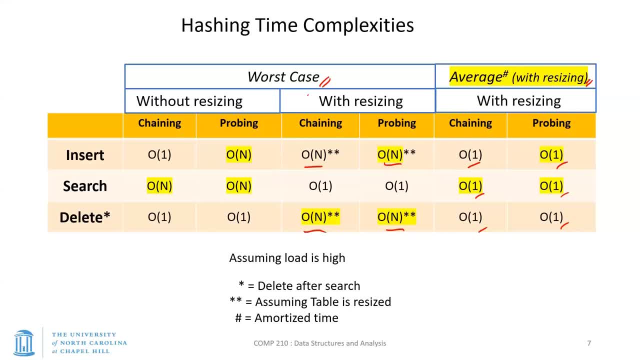 So at this point You might say: well, if hashing is so good, then what about the other data structures that we looked at, right? I mean, why did we study heaps and and AVLs? Well, heaps have their importance because they're good for priority cues, and you know that priority cues- hashing is no good for priority cues. 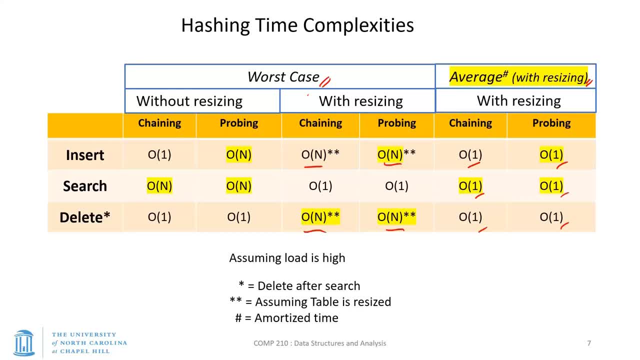 But what about AVL structures? I mean, what about BSTs and RBTs and AVLs, which are balancing BSTs? So what about those? Do we see that? Do we simply discard all of that knowledge? Probably not, right. 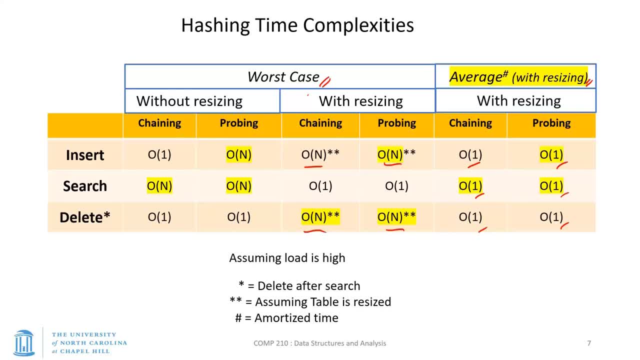 I mean, you spend a fair amount of time discussing those, So there's probably a reason why we discuss those. So any thoughts: why do you think an AVL or an RBT would still be useful? This is where you sort of look at the big picture and try to think, putting different data structures together in one perspective, and try to think what are the pros and cons? 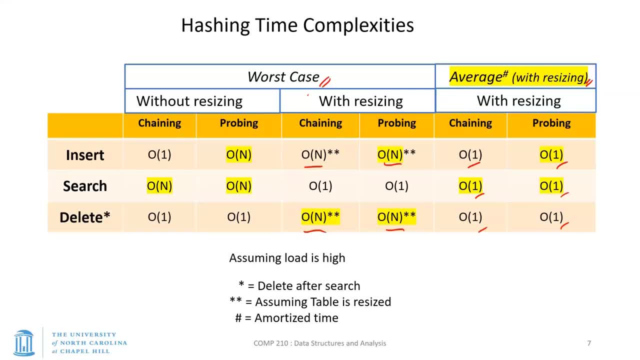 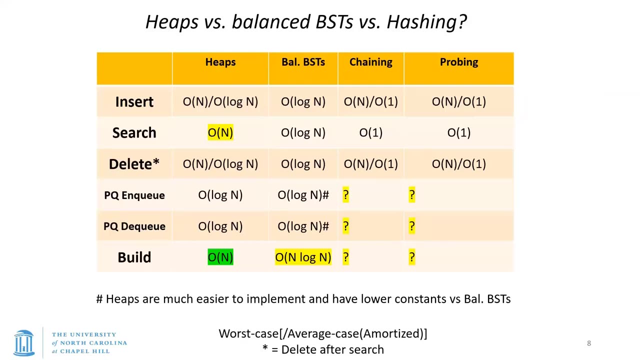 So now you have to think about applications When you think of any applications where hashing may not be looking so good. And let's now take a look at the following scenario. So this is something that we've already seen before. Okay, So this is heaps and balanced BSTs. 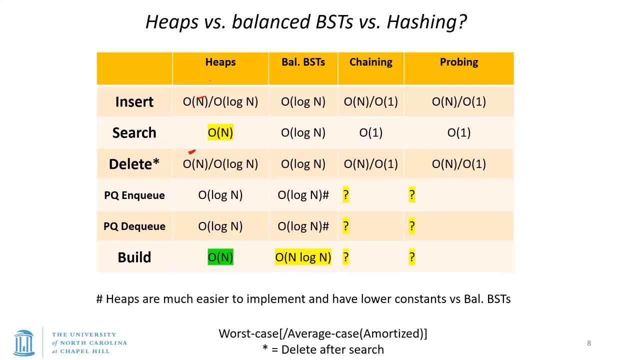 So we saw those earlier. All right, So you have a heaps structure and you have a BST structure. So you have to think about it structure. right here we have the balanced PSTs, and now I'm trying to compare that with chaining and 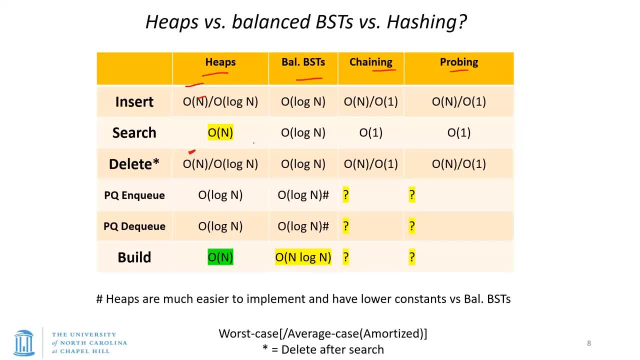 programming. okay. so you've seen, and what I'm doing is I'm putting a slash between the worst case and the average case. so where you see, uh, two numbers appearing, then it basically means that in the insertion for heaps number that we said, because it's resizing, it's going to be worst cases they. 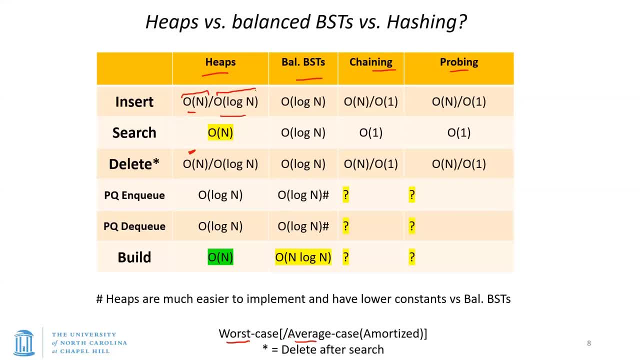 go in. the average case is going to be order plug-in. the search for heaps was always big open. why? because heaps are essentially partially sorted. it's not BST, so you have to go through the entire entire tree deletion. the worst case is big of n because it might result in a resize. 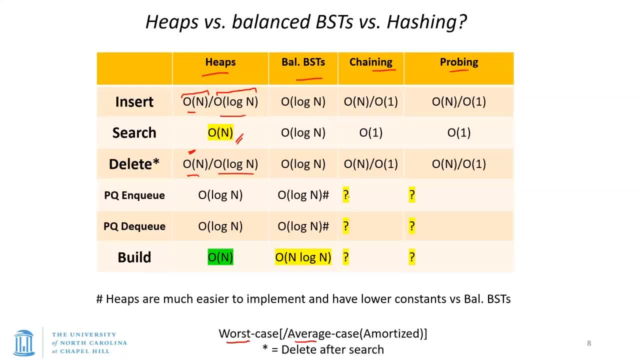 or an average. we've already seen that it will be an order plug-in. okay, uh, for priority queues. this is a great structure, okay, why? because one of the things that we saw is that the uh, the build time complexity is big of n and um, the worst case for doing a dq, and. 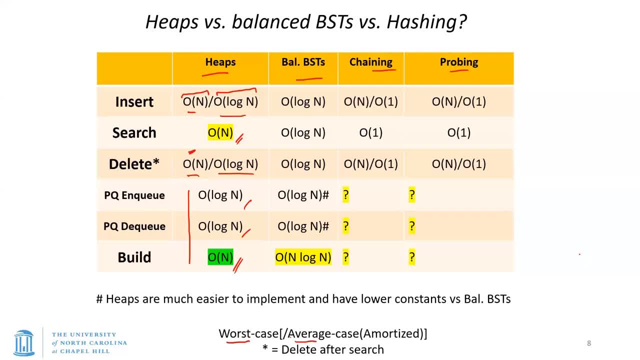 mq is also guaranteed to be order of n. order of log n. okay, um, I have that one over here, so the worst case involving this is called. so that's, that's the average. so the worst case, uh, sorry. so the worst case is going to be order of n. 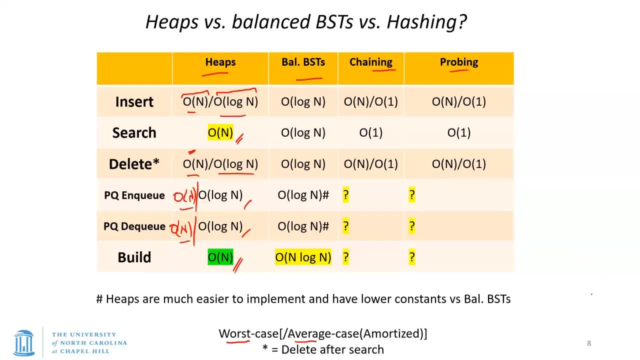 why is that? because, uh, they have to be dq, they have to be resized, okay, otherwise it's going to be order of login on average. uh, balance BSTs: we saw that they're really good if you're talking about insert, search and delete, but, um, not so good as far as build is. 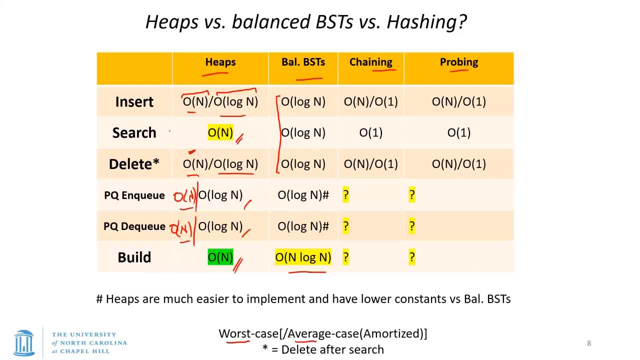 represented by interaction trade. okay, so we've gone over this portion earlier. hopefully you recall these results. and now we're talking about chaining and probing and I've just shown you that the worst case and the average is as follows for Insert, search and delete. okay now, um, we can also take a look at this, all right. 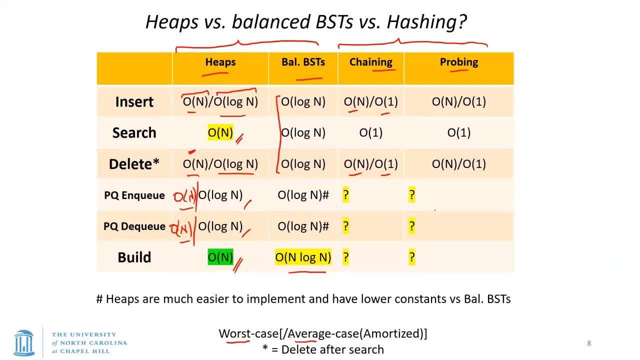 So any thoughts on if you try to hashing for a priority queue implementation, would that work out at all? could you use a hashing for priority queues with any luck? no, and why is that? yeah, yeah, so so in hash hash table there is no relationship between the location. 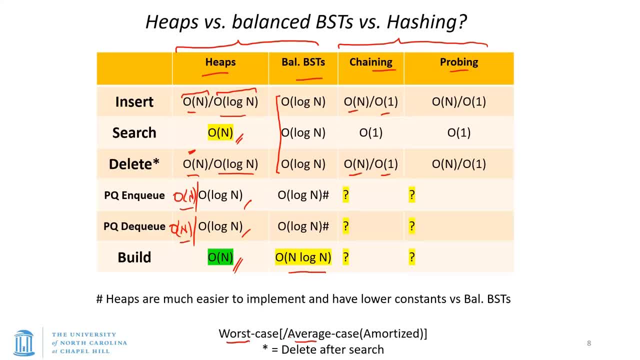 of entries, right? so in order to do a DQ of the maximum or the minimum, we simply have to go through the entire table. so that's no good. so if you look at the following results, this would certainly be big O. okay to do a DQ, simply because you would have to go. 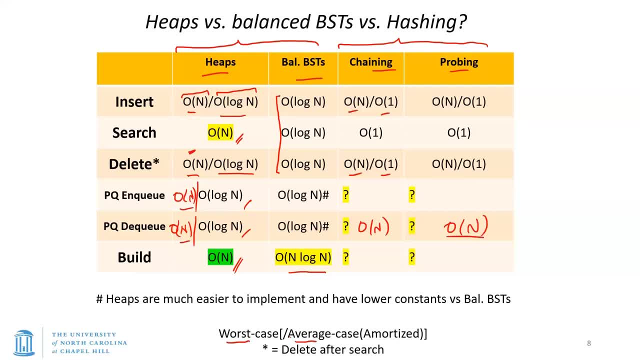 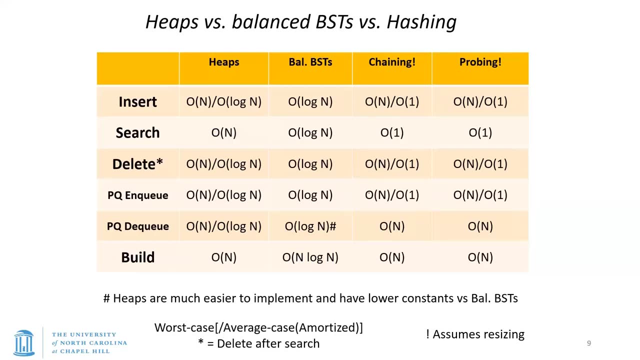 through the entire hash table. okay for an N queue again, the insertion might be quick, but the the deletion that the insertions would would result in a worst case of order of n on average big of one, uh and the same. and essentially, if you look at these two scenarios, these are: 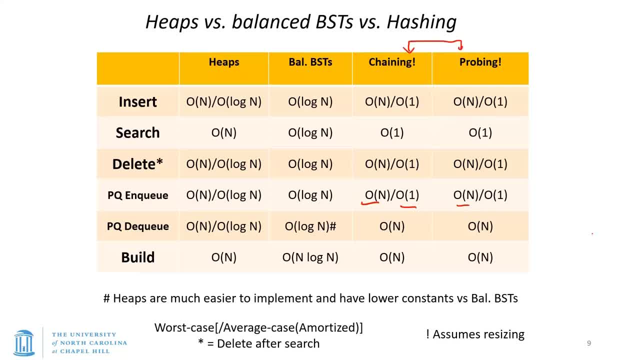 identical in terms of performance on in terms of bigger complexity, okay, um, what about build? can somebody sort of justify why I put a bigger N for a build in in hashing? so what are we doing in build? we're basically saying: all of the elements available to you, so you have n elements. now you're trying to build a hash table with that. 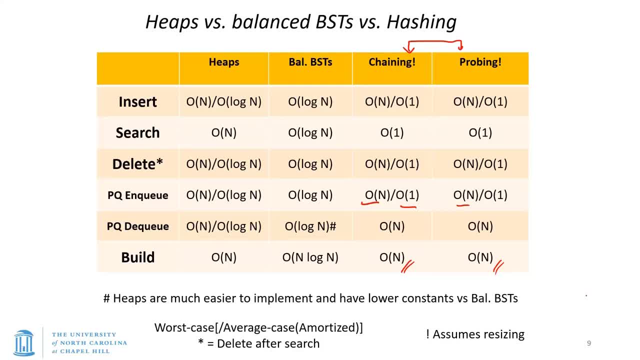 how long should that take? yeah, right, yeah, exactly. and uh, what about resizing? did you have to resize, okay, yeah, yeah, yeah, so because you already know how many elements you're supposed to add, and that's what build means. remember, so, in the build, you already know you have n elements, so you don't need to. 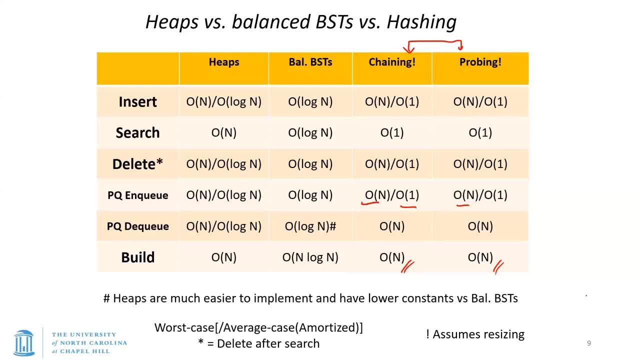 resize: okay, you simply start off by setting the user the threshold and if you're doing probing or chaining, you would use the appropriate threshold and you'd say: well, if i have 100 elements and i'm doing chaining, then i can simply take a hash table of size in 100- okay, and i simply insert those using a hash function and 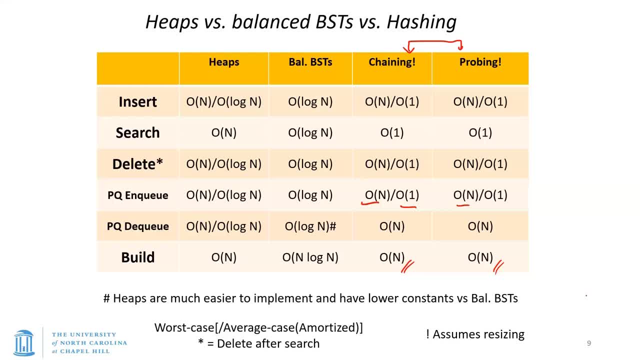 you know that's going to take all different time. okay, so you don't have to resize, okay? so that's the reason why the build operation in both of chaining and probing is going to take bigger time, okay. well, we've already seen why this would be big of n, simply because, um, it's going to be dq. 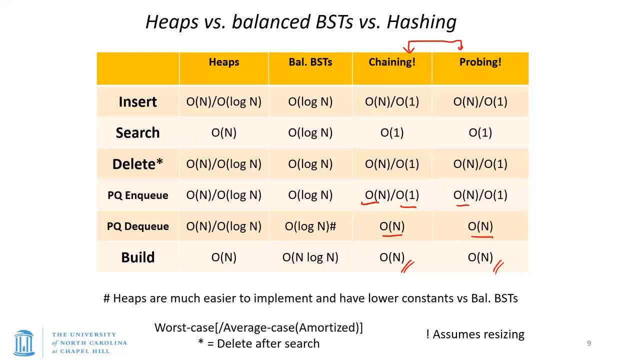 and there is no relationship. so you simply have to search through the entire hash table to be able to find the largest or the smallest element to dq. um, if you're doing an nq, the worst case is that it would have to be resized. okay, both of these cases, but on average it's going to be order of one. 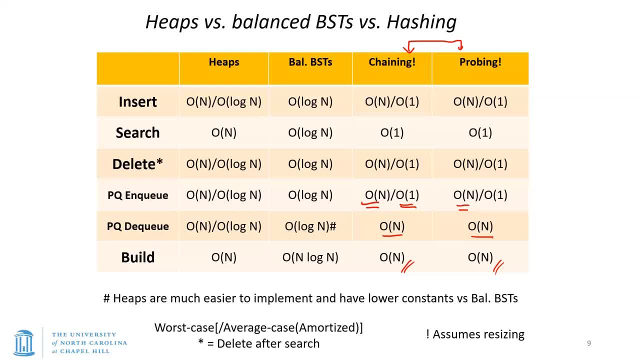 why is that? because we're talking about amortized values, so it doesn't really the resizing doesn't matter, and so when you're doing an nq, either in chaining or probing, it's going to be a constant time as long as you're doing resizing. so we. so here, in these two scenarios, we're going to be. 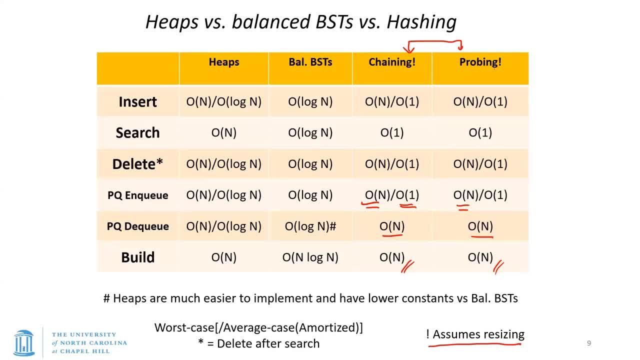 assuming resizing. okay, that's what the estimation comment over implies. okay, so this is sort of uh a good point to sort of try to see, well, which one of these uh data structures would be used in what scenarios. okay, and um, you can see that in some of these uh for the priority queues, uh, which one would you use? 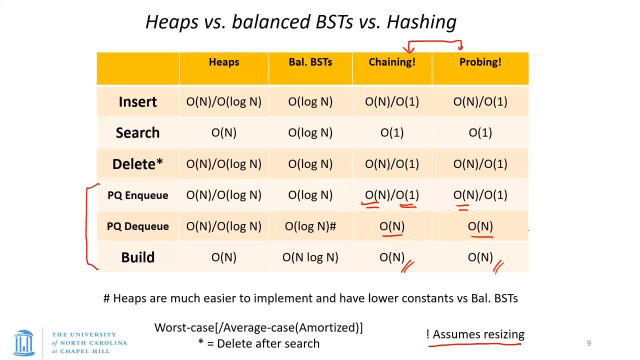 you certainly can't use uh hash tables, the priority queues, simply because of this particular problem. right, there is no relationship, but uh, we've already discussed this. for just a review. if you want to use a priority queue, could use a balanced bst versus a heap. we could, but there is a little bit of an advantage for a heap, simply because using 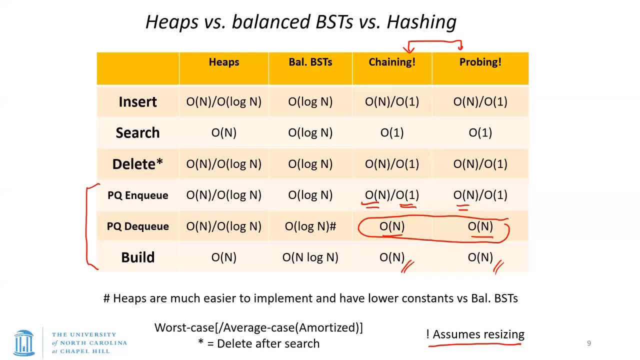 a matter list, right, and a balanced bst would be using arrays, so i would be using pointers. okay, and if you're using pointers then you're obviously going to take up. you know, the constants associated with the log n are going to be larger, okay, so the heap. 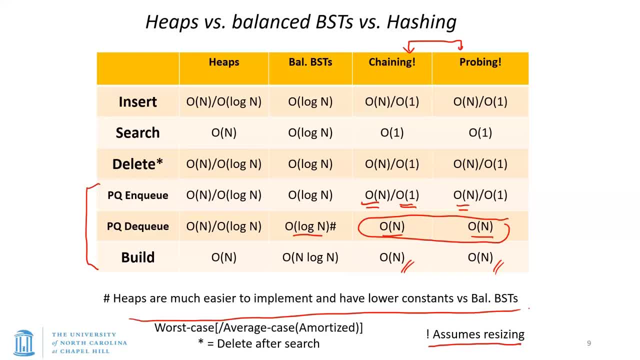 is going to be much easier to implement and have lower constant. so we've already discussed this. so, as far as the priority queues are concerned, uh, heaps are great. um, as far as doing insertions, search and delete, it seems like if you're talking about averages, then hashing would be the best way. 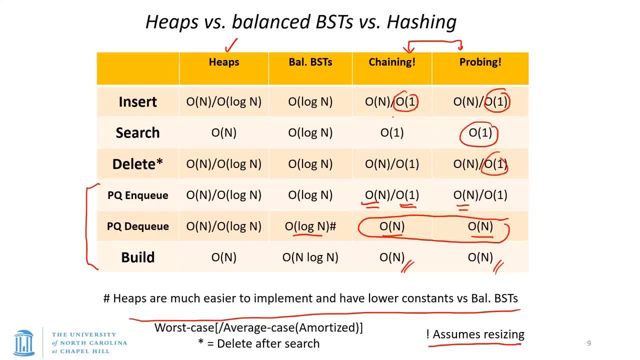 to go all right. we're talking about averages, so where does our balanced bsts come in? can we see any use for balanced bsts anymore? they're no good for priority queues. they're no good for priority queues. um, they're not the best. they've been superseded by hash functions for doing the usual insert. 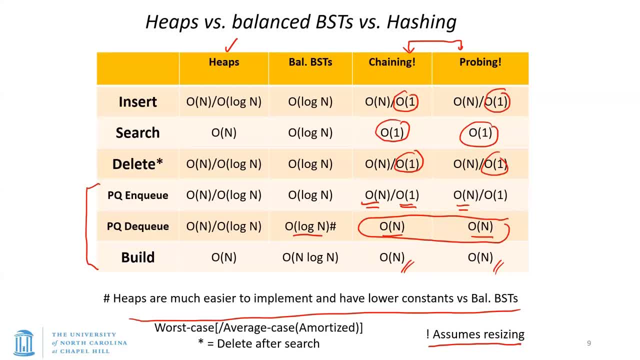 search, delete, but can you possibly think of as an application where, um, honesty, bscs might still be useful, even for your insert, search and delete functions? yes, okay, so if you're doing a lot of insertions and deletions, then, um, well, even then, on average, 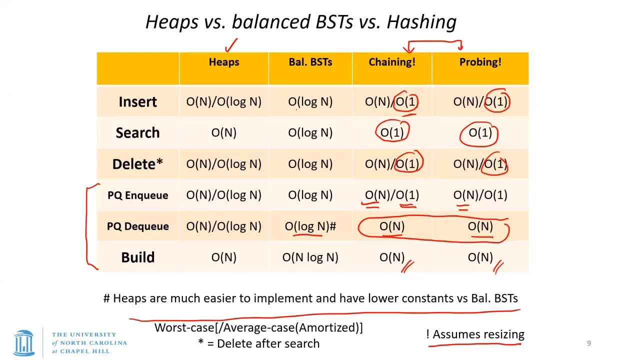 hash functions are superior because insertions and deletions in bsts are taking order of log n versus on average. um hashing is taking big o of one on average. so can you think of an application where you're using numbers a lot? okay, that is um not quite sure, uh, where that is coming from, because 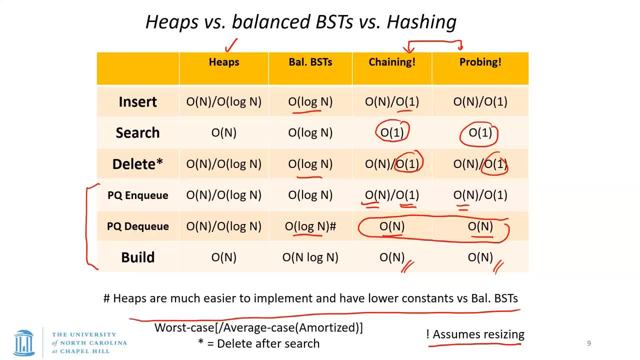 regardless of whether you have you dealing with numbers or you're dealing with a string to compute, a hash function is going to be a constant time operation. okay, so, numbers versus strings or objects, uh, the hash function is going to be equally good, at least in terms of complexity. 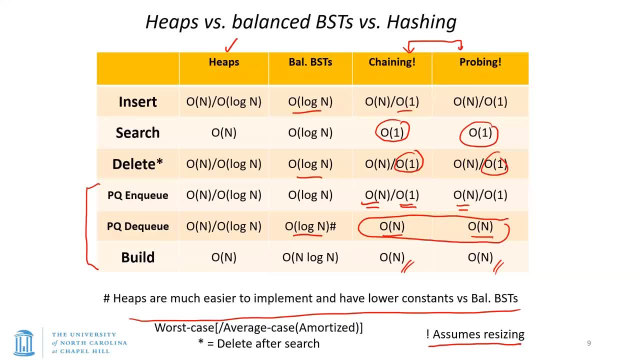 okay, yeah, i can see that. so, depending on the application. so here is a general way of thinking, thinking about this: if you are running a real-time application, okay, so imagine that this um application is actually being used inside a self-driving car. right, you are going and you see a red light and the car is supposed to stop, right, all of a. 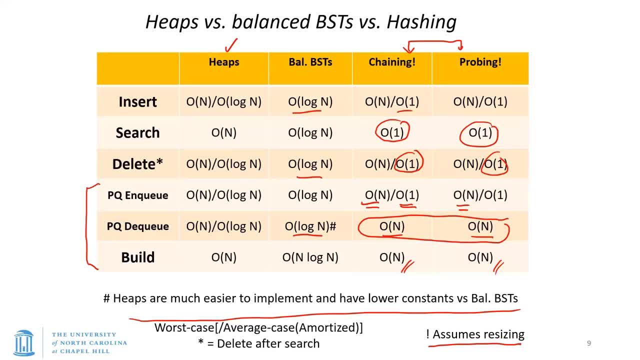 sudden, the information that's coming in requires that the table is to be resized. what's going to happen? it's going to take a huge amount of time. it's going to be an order of n operation. uh, in that particular scenario. so an average. your car runs fine, it goes through all the green lights. 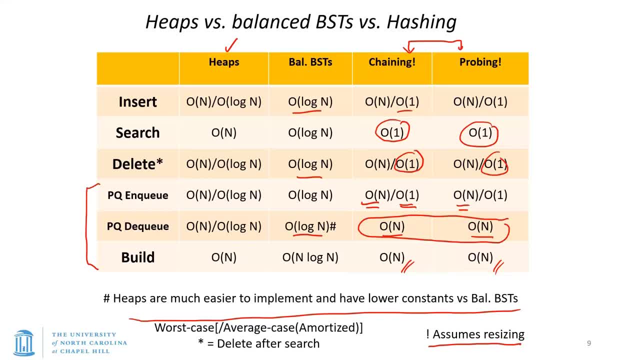 and red lights. but on that one particular day, uh, you went through, you're going through a particular scenario and all of a sudden, you're seeing a resizing happening. what's going to happen? you're going to go to the red light. you might actually, you know, have a major problem. okay, if you get a ticket, it could be a lot worse, okay. so, 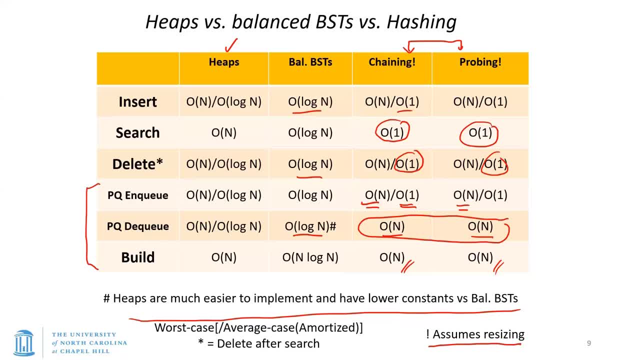 in all the real-time applications, you need to worry about not just the averages, but you need to worry about the worst case. so if you are running, uh, an application which is a real-time application, it will be safer to go with the balanced psts, even though the 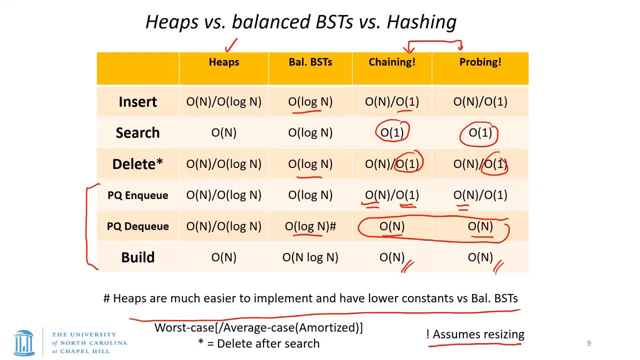 average performance for a hash is not superior, which is a big of one, as compared to a balanced pst which is over log n. okay, but at least are you. it's predictable, okay, um, and you have this unpredictability whenever you're using an error list and you don't want that kind of a situation. 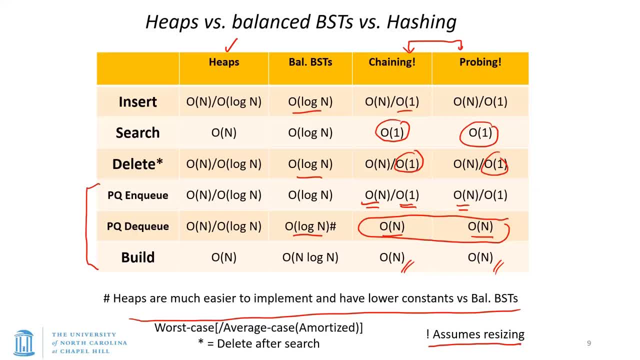 coming up if you have a, a real-time application. okay, so now you can see that you know all of these have their pros and cons, but there is, uh, one thing that seems to be- there was a question earlier on- and that is: i mean, why are we using probing versus chaining? right? so we come back to that particular. 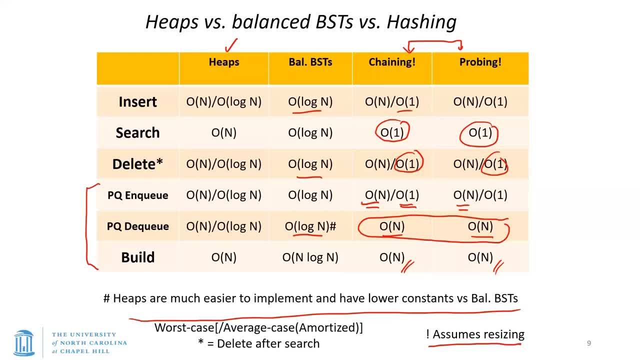 question, and it seems like probing and chaining are performing identically, um, in terms of the um, complexity, but, uh, what seems to be the difference, and can we just uh think about, is, you know, the threshold for chaining is superior in the sense that you can have a higher threshold before you. 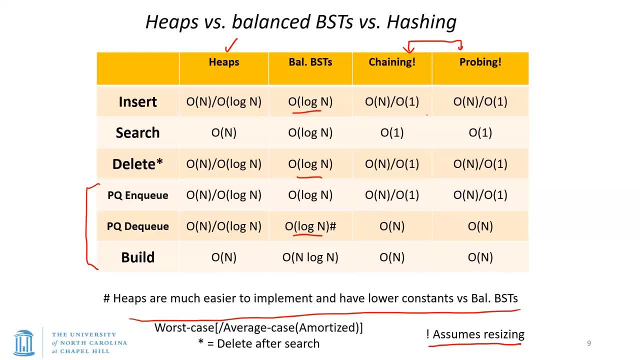 resize or probing doesn't look so good in that respect. so why, uh, do we need to worry about probing versus chaining? what could be the pros and cons over there? so it's clearly not in terms of the complexity okay, because in terms of the complexity, the bigger notation. we're performing identically. 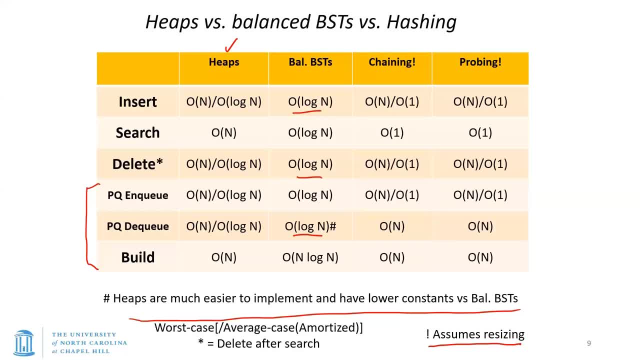 so now we're looking at something a little bit, you know, slightly different, maybe in terms of the constants, or maybe in terms of something else. yeah, yeah, so, so you might say that in chaining you're actually using two data structures. okay, so you not only have the? 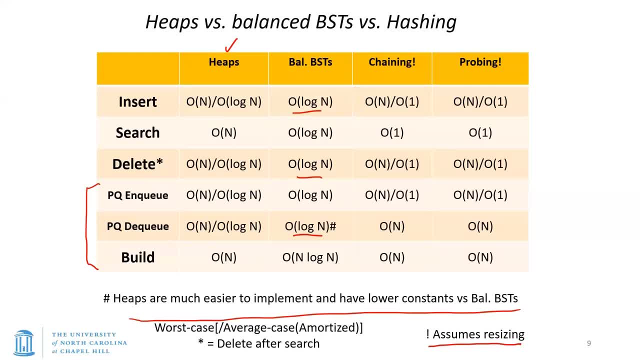 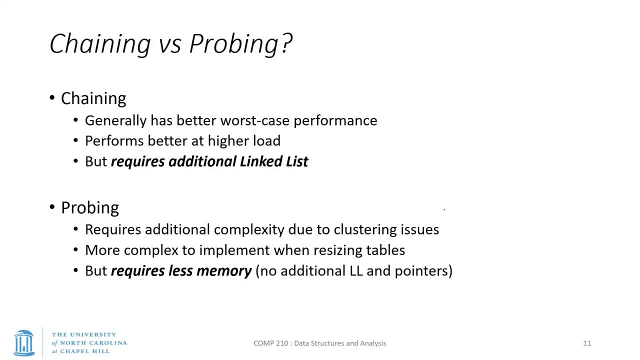 array list, but you also have to have um, a linked list, okay, so it's more complex. so you might be able to summarize this as follows, and this is some of these results. i'm not really proving to you, but generally chaining has been seen to have better worst case performance. okay, so it seems to be good. 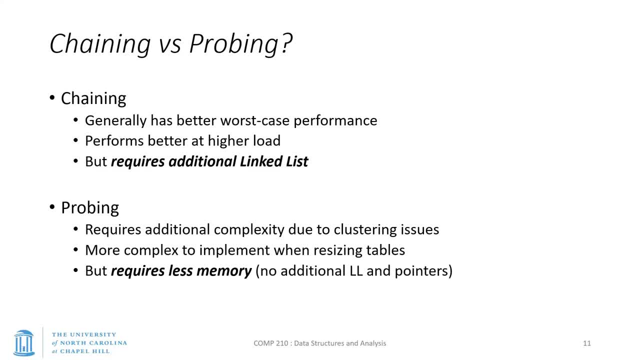 uh, it also performs better at higher load. we've already seen that. but in probing it's a little bit more complex because the threshold uh is higher for chaining versus probing. however, uh, it does require this additional interest. okay, so that's a bit of a you know. 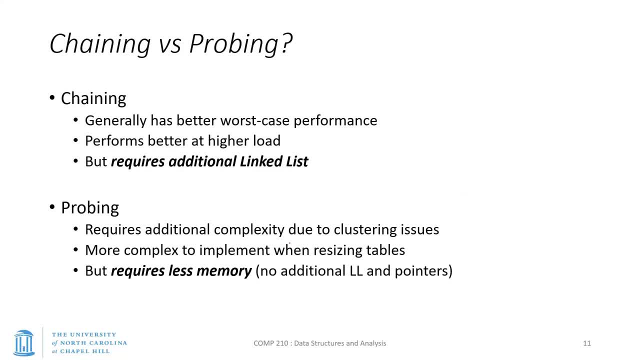 trade-off in probing uh it. it requires additional complexity due to clustering. so you know that you've got to implement double hashing. so, uh, if you have a problem and you have two manipulations, you've got to have that cluster. then you've got to have, you know, some nice complex uh. 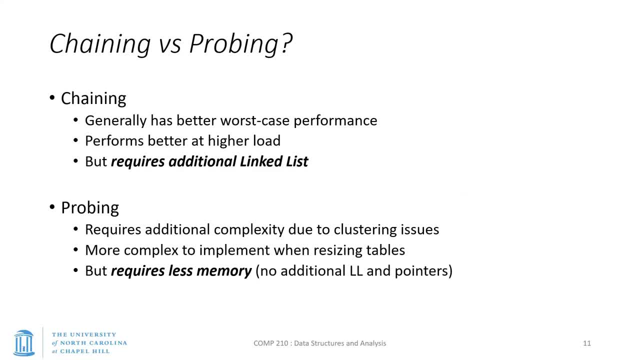 hashing functions to be able to avoid the clustering issue. um, it's also more complex, okay, to be implemented because of the resizing, so underlying, there is a resizing issue, uh, and you have to actually copy everything. okay, um, however, but of course, this particular issue is also there in in chaining, because you would have to resize. that all right, but 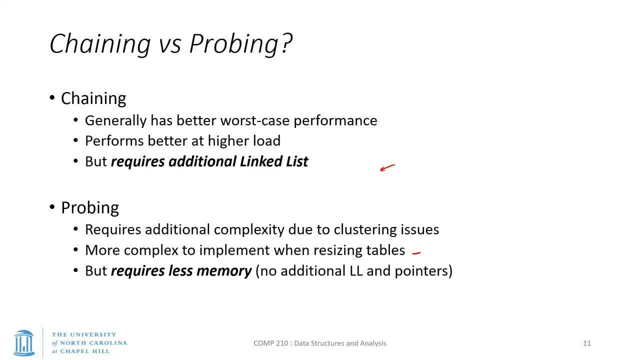 in general, it requires less memory. and why is that? that's simply because the linked list has pointers, so it's the fine print, right? there are some advantages to both of these. so if you are concerned about memory, you would go with probing, okay, so if you want to make it something, 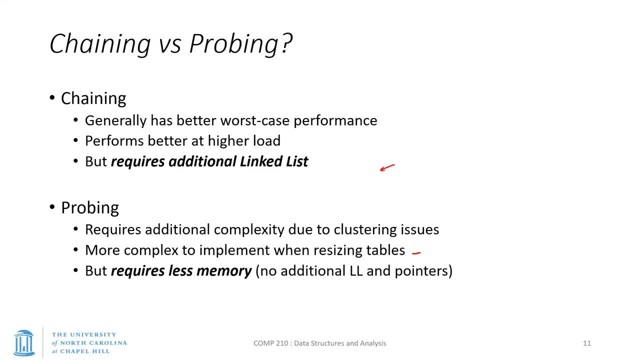 um, simple, and you don't have to worry about two data structures and have to worry about, you know, managing the linked list. uh, then probing works fine, okay, so there are some fine uh differences between these two. so this sort of uh brings us to the end of our data structures, okay, and this is an important. 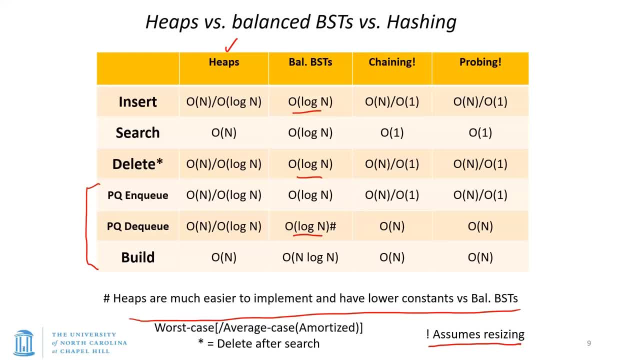 table, because it basically- uh, you know- summarizes most of the results. uh, not for stacks and queues, but for pretty much everything else that we've discussed. this is a good point to review the entire course after this stage. all right, so now we will move on to the second part of this course. 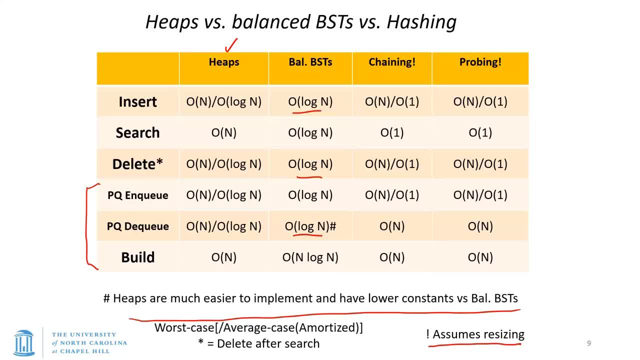 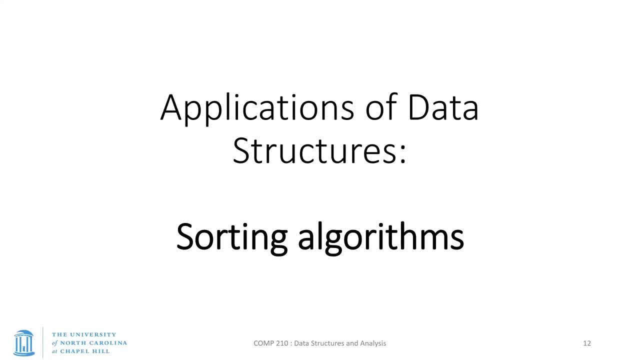 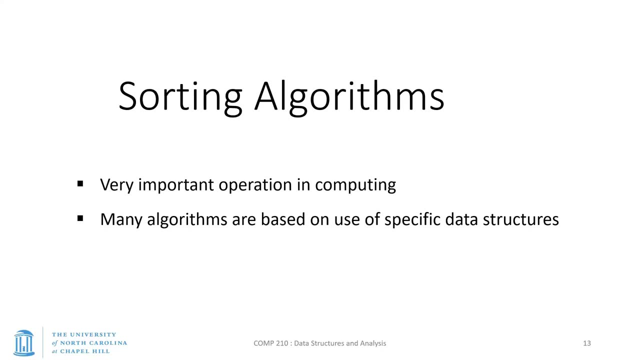 which is talking about application. okay, and the first application that we will start talking about is sorting algorithms. now, uh, sorting algorithms is something that we've sort of- um, perhaps thought about right from the stage where, you know, in the first or the second lecture, where we were saying that, um, well, if you're trying, 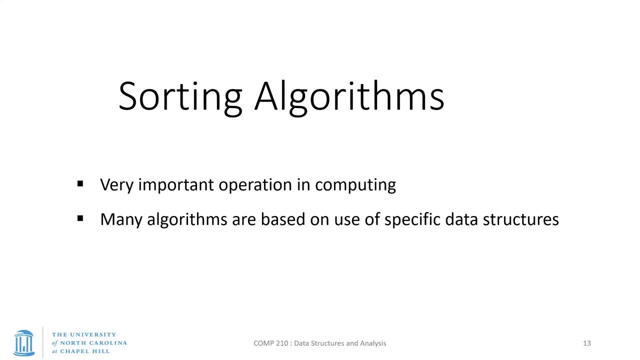 to search. what is the first algorithm that we taught, which operates, you know, in order of login. i think that is in the second lecture. how could we, yeah, find research? and what did we say about binary search? we made a big assumption. we said that if, if the data, yeah, is sorted right, so right away, we're saying that if the data was already sorted. 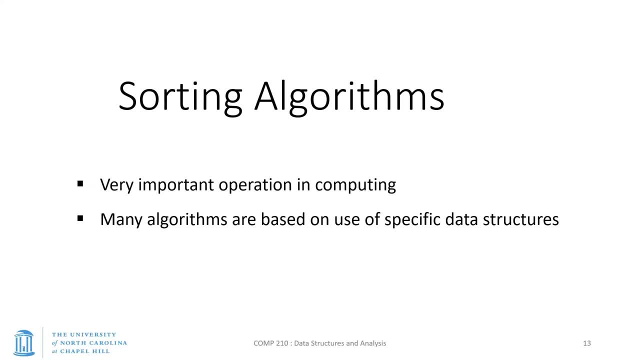 we didn't say how it's going to be sorted, but if it was sorted then we could do a binary search. so you can see that, um, having data sorted is extremely important and you know you deal with it every day, every time you open your your phone book or something. it's all alphabetically sorted, right. 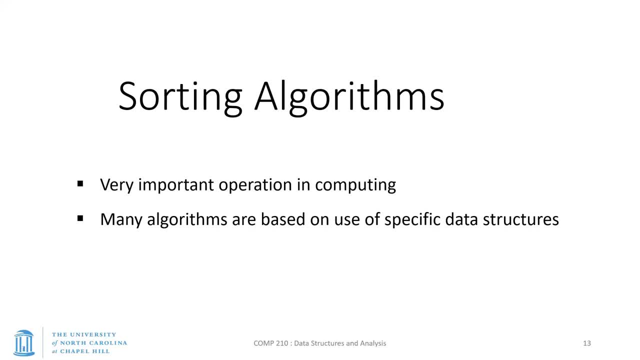 uh or your phone numbers or what have you. so sorting is one of the important uh applications that is used throughout computer science. all right, it's very important. computing in general, um, now, in sorting, um, what we'll see is an application of data structures. now we'll see several sorting algorithms. some of them have nothing to do with data structures. 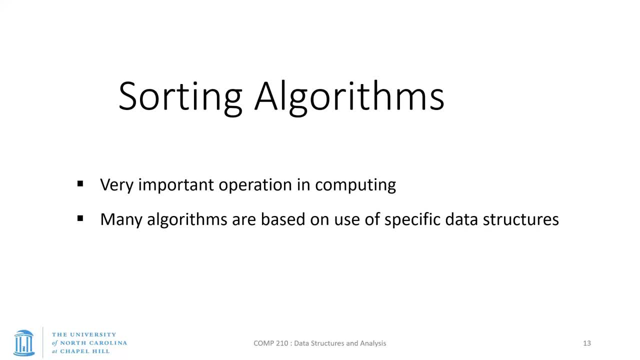 those will be starting points. so we'll say, well, let's assume we learn the data structure scores, let's see how we can actually do some sorting, some simple sorting. and then we'll finally say, well, what if we try to use some of the data structures that we've already studied? can we improve on the details? 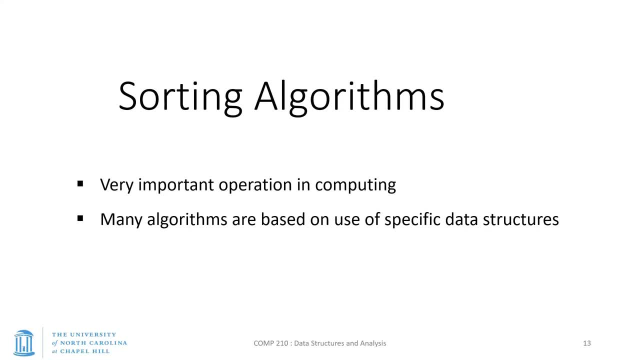 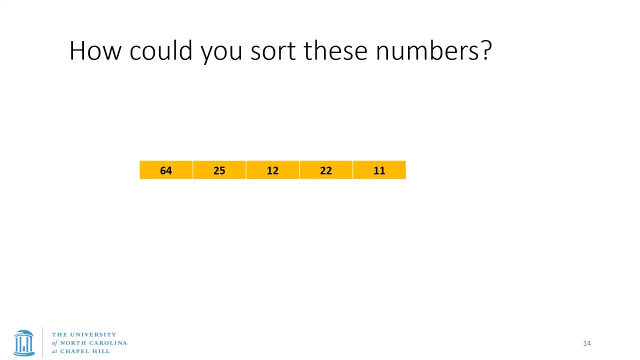 interestingly. yes, data structures does help. okay, So let's take a look at how one could sort, And for now, for the next few moments, we'll forget about data structures for a while. okay, So let's think about how, if you had a bunch of numbers, 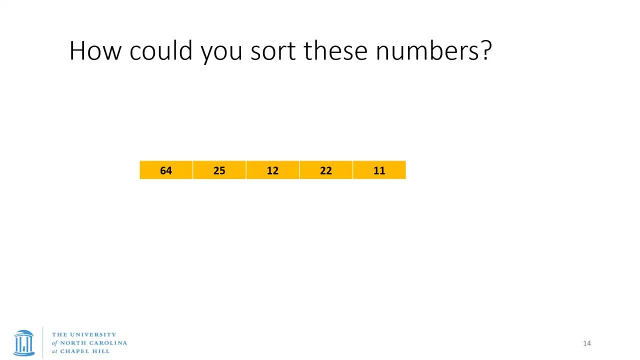 okay, in a really simplistic way, just maybe cards, nothing to do with computer science, and you had to sort these okay. So imagine that these are pieces of paper that you have to sort. How would you actually go about sorting them? 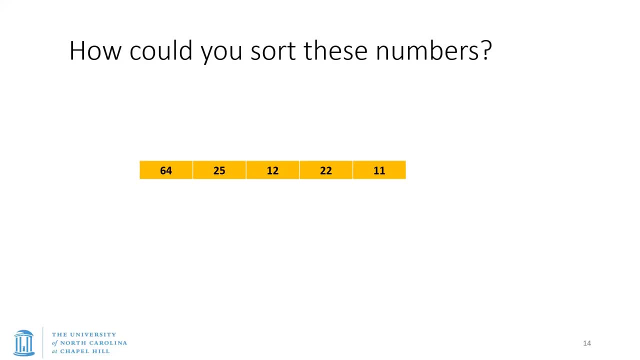 Any algorithms that might come to your mind. okay, Don't think about computer science for a minute, okay? So somebody who's on the street and you ask them: we have a bunch of numbers. how would you sort these? And we do this quite often if you play cards, right? 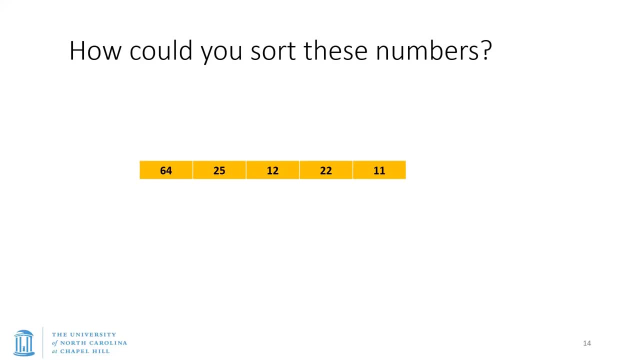 You have a deck of cards and you need to sort them. so how do you do that? Yeah, Okay, Okay, that's a good algorithm. So you could say, well, 60-4,. you compare these two and you say, well, 25,. you kinda sort. 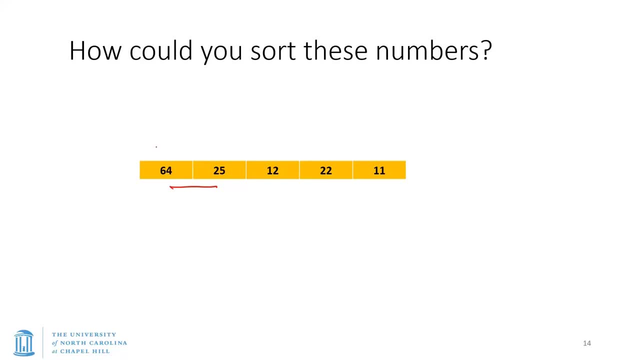 with the largest number on the right. So you say, well, let's move 25 over here and let me do that at the bottom. So we move 25 here and you move 64 here. okay, And then perhaps you do the same thing. 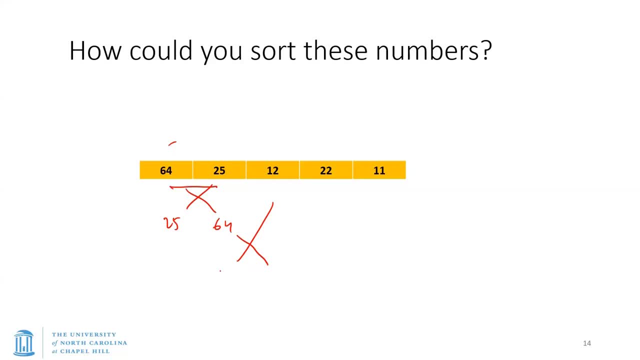 You compare 64 with 12, right, And you say, well, 12 should go down, 64 should go up, and then you keep on going in this direction. is that how you do it? yeah, so you'd have to do to go through it multiple times, right, because we already 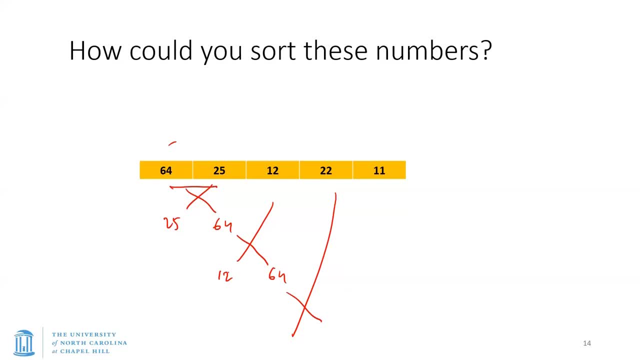 see that, even though these two are relatively sorted. but over here we have a problem: right 25 is still bigger than 12, so you'd have to go through a second recreation through the entire process. yeah, okay, so. so in that sense you would have to first of all say which is the highest or which is the lowest right. so 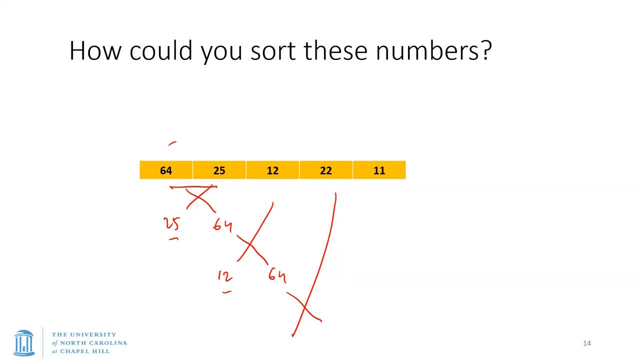 in that case. so that's an alternative. so these are two algorithms that we write about a study in the next few minutes, okay, the first one is called bubble thought. okay, what you just suggested, that's what about it. so, basically, you're doing a comparison, okay, and you sort of doing a comparison with neighbors and 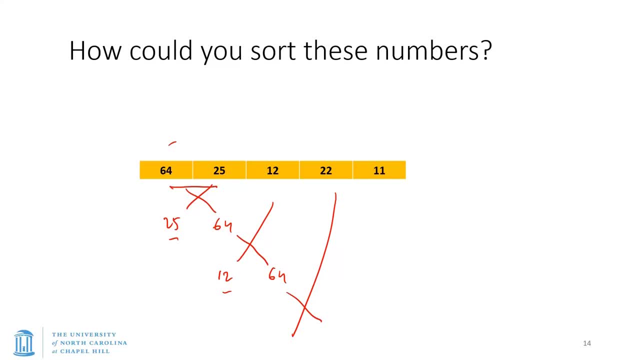 you, you swap them, they're in the wrong order and you go through the entire list once and then you do the process again. okay, that's public. so the other one that you just suggested is saying: well, what if we go through this entire process and we find the largest one? okay, and then we put it at one end and then we go through. 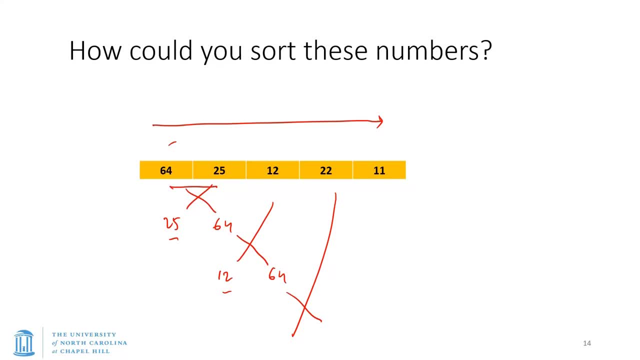 it again and find the second largest one, okay, and then you do the process again in order to get the last one, and then the second last part, okay, and that's called selection song. okay, so these are two, the roughly these are two algorithms, okay. so the first one is Selection sort that we study and then we'll talk about. 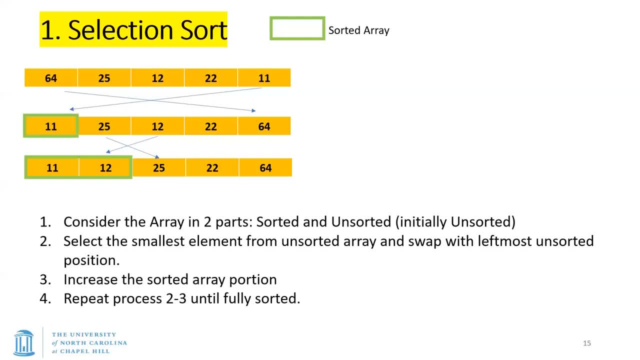 bubble. so ending next month. so selection sword basically says: well, we will separate this array into two components. okay, we'll say, well, this is some portion of it will be considered as sorted, which I'm showing a green box, and the rest of it is unsorted. okay, so consider the array in two parts, sorted and 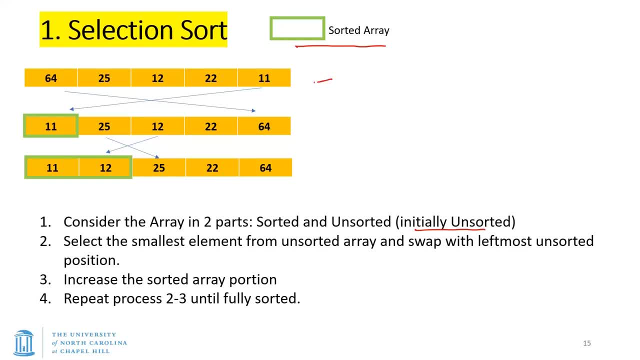 unsorted. initially, everything is unsorted, so there is no green box over here. the second step is select the smallest element from the unsorted array and and swap it with the leftmost unsorted position. okay, so now we're going to go through this entire array and let's. i didn't say this. 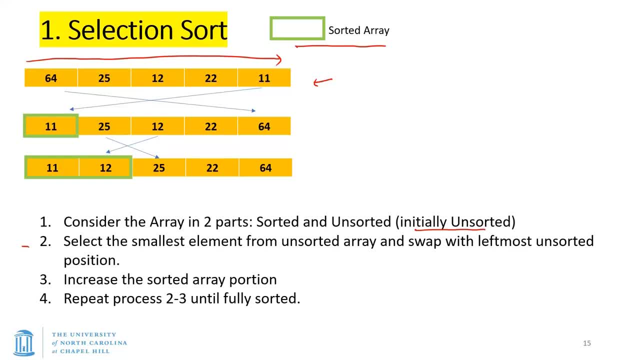 but let's assume that this is in some kind of an array, maybe a static array, okay, so we're going to go through the entire array and we're going to look for the smallest chart. we find that 11 is the smallest. so what are we doing? when we're doing the comparison, we probably have a variable which 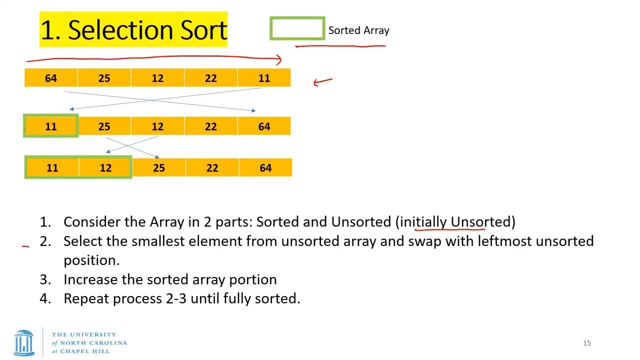 says this is the current smallest one, and we initially have the variable saying 64 is the current smallest one, and then we go to the next one and say, well, 25 is smallest. now the smallest number is 25. then you say the smallest number is 12, and then we say the smallest number is: 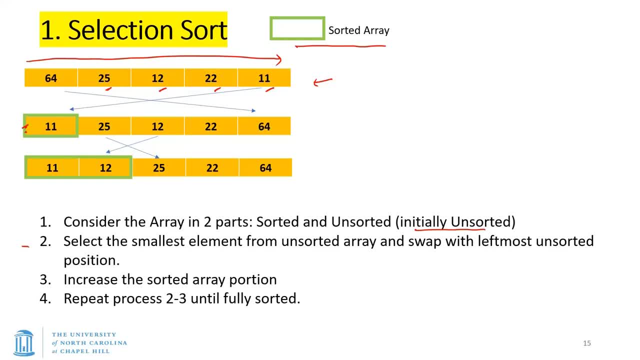 still 12, and then we finally get to 11 and we say: now the smallest number is 11.. so now we found the smallest number, and what do we do? we swap it with the first location, okay. so 11 comes up here and 64 goes over here. one iteration done, and then we continue on from this point onwards, okay. 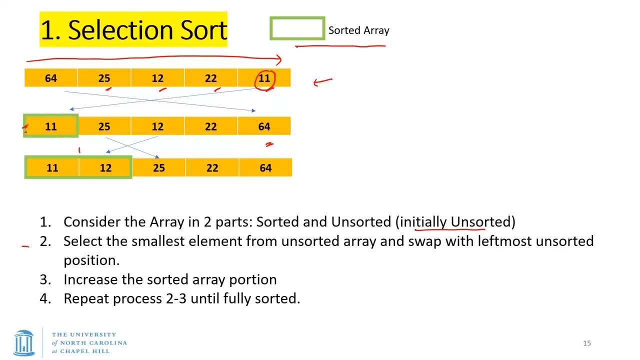 increase the sorted array portion. so now the sorted array portion is increased and now we're going to repeat this entire process for the rest of the unsorted array. so what we do now we look for the smallest number. so we look at 25. this current smallest, now 12, is the smallest 12 is 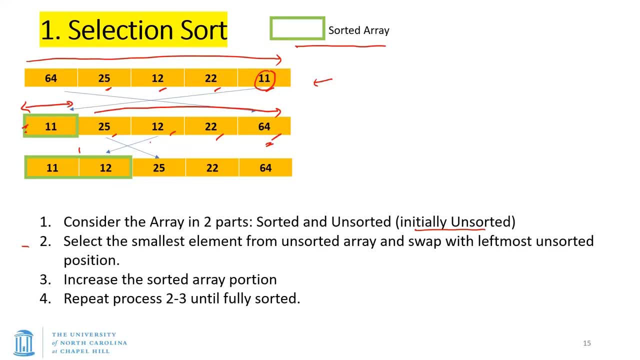 still the smallest. 60, uh, 12 is still the smallest, so now we swap 25 with 12. okay, so now this portion is sorted and this portion is unsorted, so you can see where this is going. now let's try to compute the complexity and we look at the worst case, the best case and the 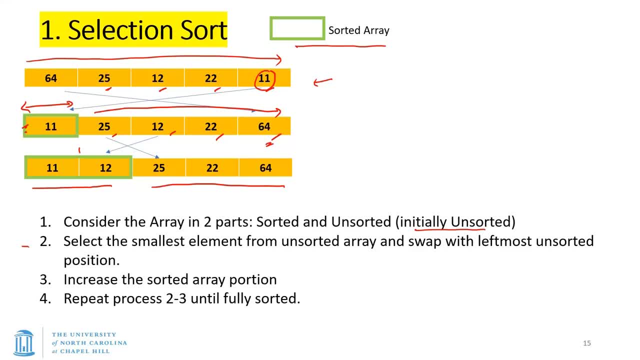 average case. so the average case is generally difficult because it requires probabilistic analysis, so we'll simply look at the worst case and the best case. okay, so let's think about the worst case first. okay, what is the worst case performance in this scenario? yeah, so o of n is one answer. 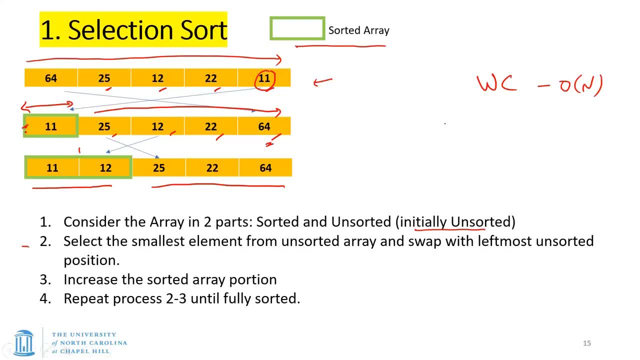 um, any second talks? yeah, yeah, yeah, see, the first time around you're going through all your n n steps right. the second time around, in the second iteration, you're going through n minus one steps. the third time around, you're going through n minus two steps. why? because 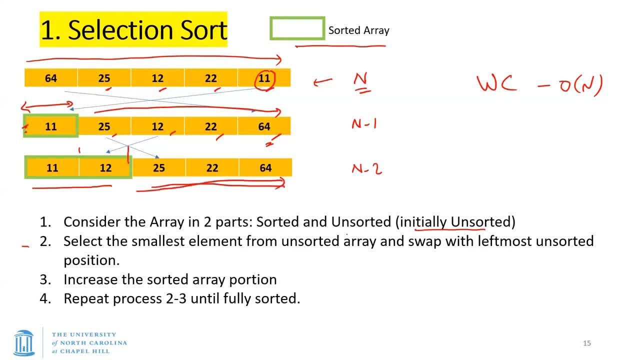 you've already sorted this portion, so you're only going through the rest of it. so the number of steps is going to be a sum of n plus n minus one, okay, plus n minus two, all the way up to one. and does anybody know what that sum leads to? 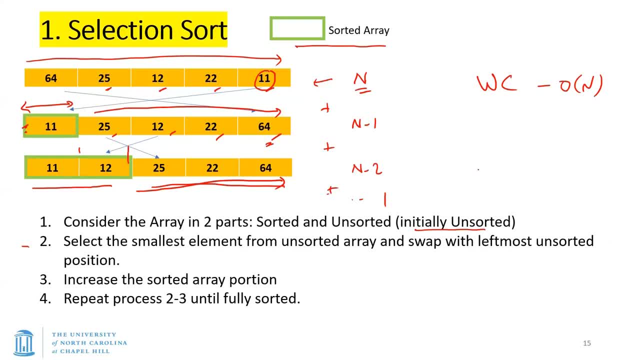 sorry. factorial, did you say. factorial is when it's multiplied, it's not as bad. factorial is like two to power n or something to power n, it's not as bad. but yes, the answer is order of n squared. but why? that simply goes back to you, know your your math. so if you do the sum, it comes out to be n times n. 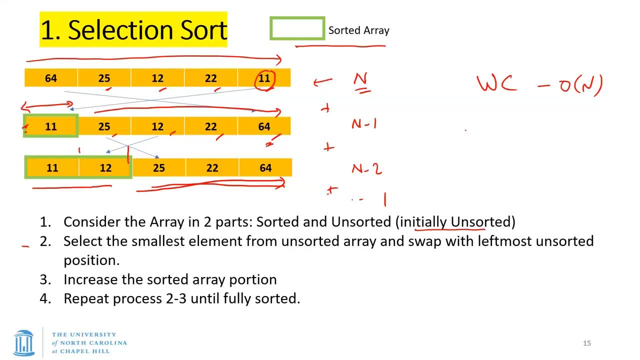 minus one divided by two, some equation like that. but basically it's an order of n squared. okay, so this comes out to be order of n squared in the worst case. okay, it's simply a sum of all of these. what about the best case? yeah, okay, so, um, that's a great idea. how do you actually know that it's sorted? so what you're doing is: 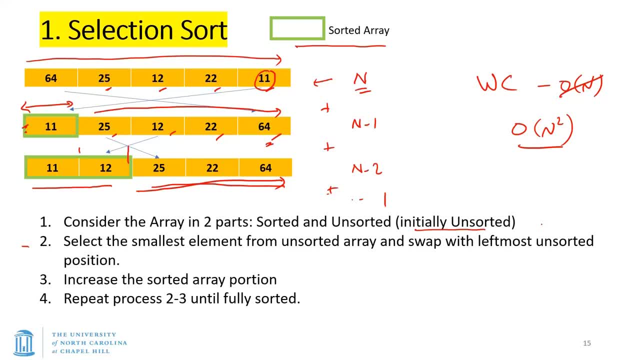 you're looking for the smallest number, right? okay, so let's assume that these are already sorted. so we have one, two, three, four. let's say we're sorting these numbers right. so now what we're doing is we're doing is we're looking for the smallest number in the first iteration. okay, you find one. you say: 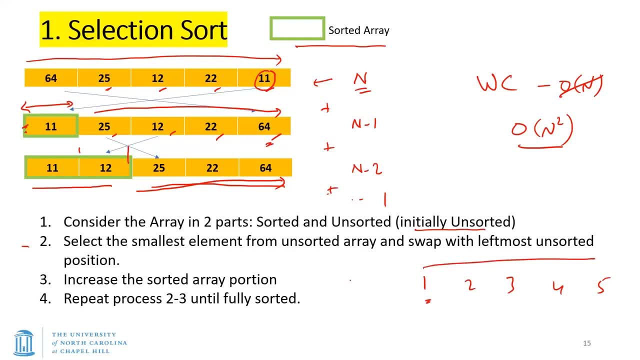 great, but we had- we had to do n steps to be able to figure out that one was in fact the smallest. the first number, yeah, it's still n squared right because the the if you look at the operation, uh, we're saying, well, one is still, you don't have to swap anything. but then you start for the rest of. 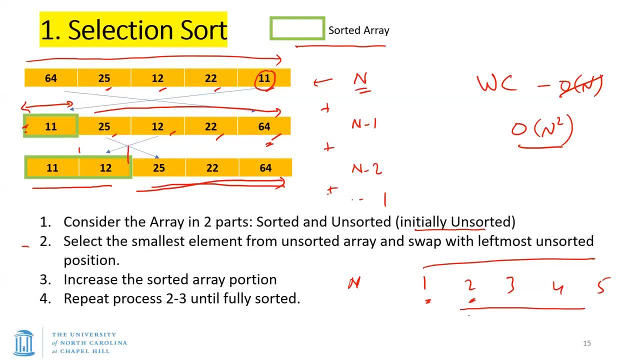 it and you say, well, let's take a look at two, and two is still the first element every time is still the smallest. but you don't really know that it's sorted right unless unless you modify the algorithm. all right, you could modify this, and that would be implying a modification of the 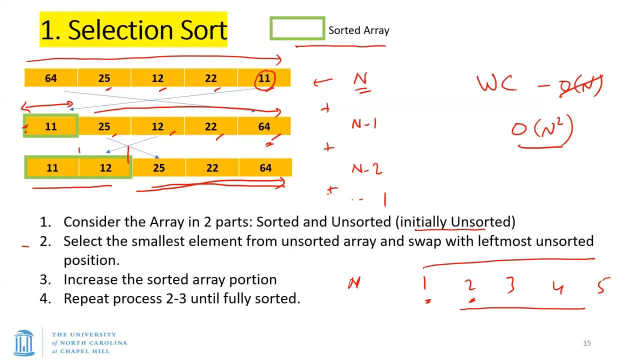 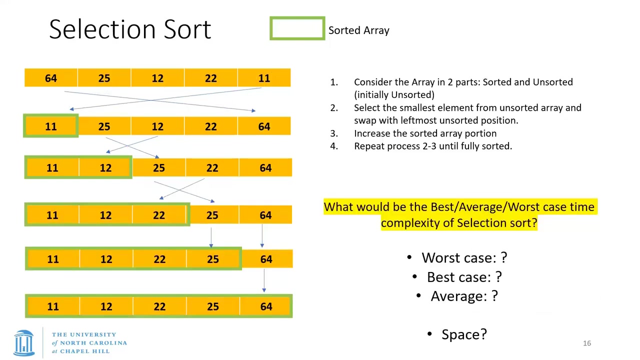 algorithm. so the original algorithm by itself would still be, even in the best case, would be already sorted. we still are going through n, and then n minus one, and then all the way up to one. okay, so this is obviously not a very good algorithm. right n squared um in both of these cases. 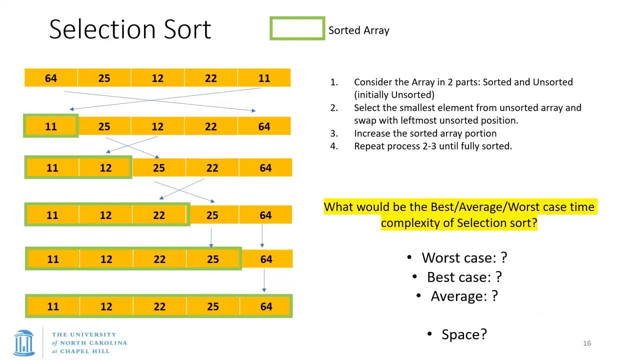 now we're also going to look at when you talk about sorting, we're also going to look at the space. and there are two ways to look at space: um, and we're going to classify the algorithms as in in space or using more space. okay, so if the algorithm is not using any additional space, which is 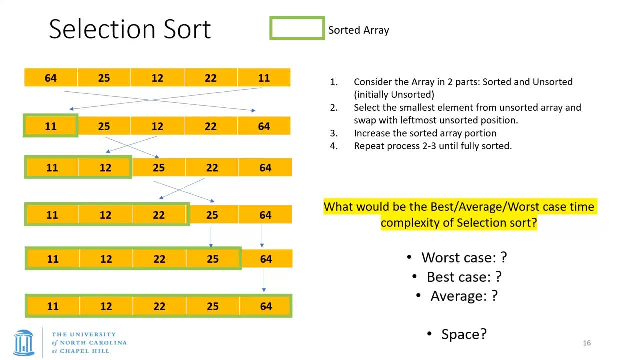 proportional to n or which deals with n, then it's going to be using- you know it's got- it's going to be using, it's not going to be using additional space, okay. so the question here is: uh, how much space is it using? additional space which is proportional, which is a function of n? 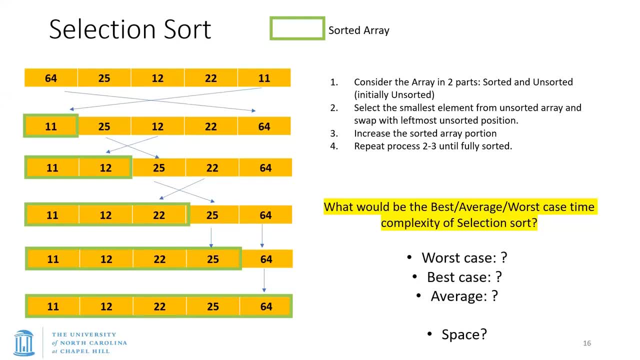 is it using additional space, which is a function of n. it could be using some additional space, but those could be fixed and maybe they're not proportional to one. they're not. they have nothing to do with n. how much space is it using? so, basically, what we're doing is we're using the array and we might have a cons, we might have a. 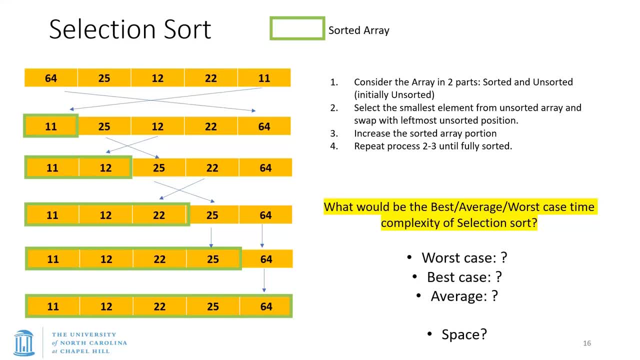 variable which is being used to figure out which is the smallest number, but that has nothing to do with them. right? that's a single variable and we're doing swapping within the array, so we're not using a whole additional array. okay, so this can be cut off as in place. 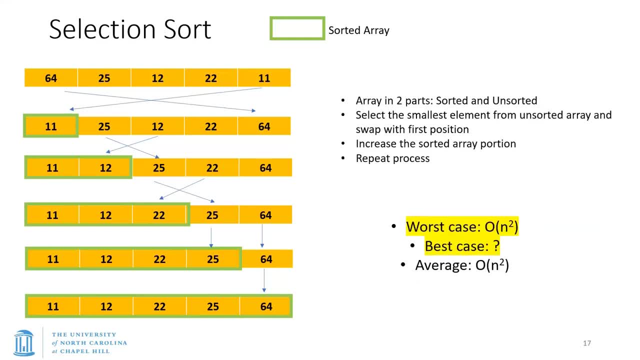 so it's really good in terms of using space, all right, um, so i've already gone through this case that you are talking about here, about. you know, even in the best case, it's going to be taking order of m squared on average. i'm not going to do this analysis, but you can see, you can perhaps guess that it's going to be. 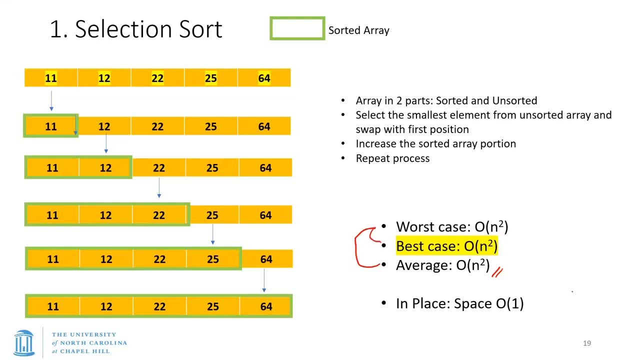 in between these two, which obviously is order of n, squared as well. okay, and in terms of space, it's considered as in place, which basically means that the amount of space that you're using is a constant. so the only thing that's going for this algorithm is that it's in place. 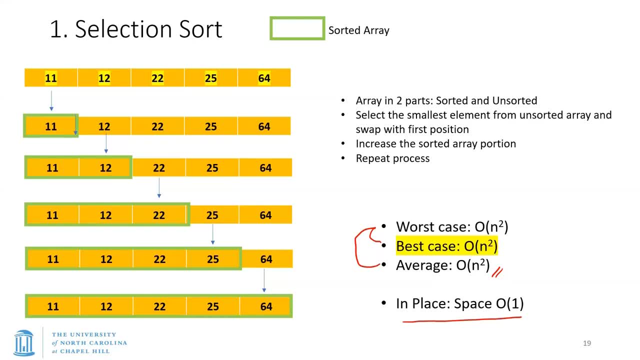 okay, otherwise, uh, it's pretty pathetic. right, it's just taking order of n squared time, all right. so, uh, that's what we normally do when we you know, if you have a bunch of cards you might be doing it that way: you're looking for the smallest number, you put it in front and then the 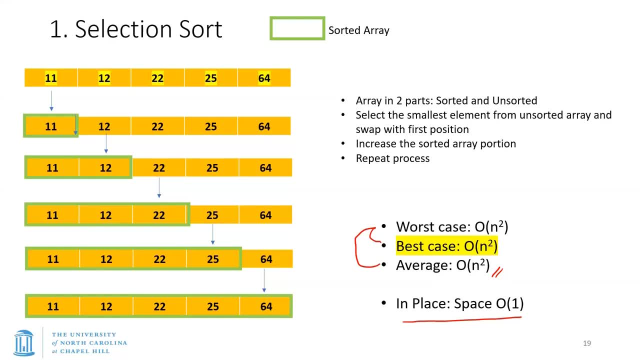 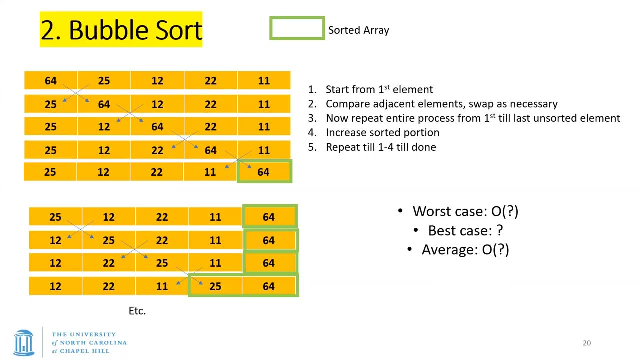 second smallest number you put in front. but you can imagine that you know the deck of cards. that's fine, but if it's something bigger it would be a problem. now let's think about the second, the other algorithm that is proposed, which was bubble sort. okay, so this goes back to one of the suggestions over here which basically says: well, let's 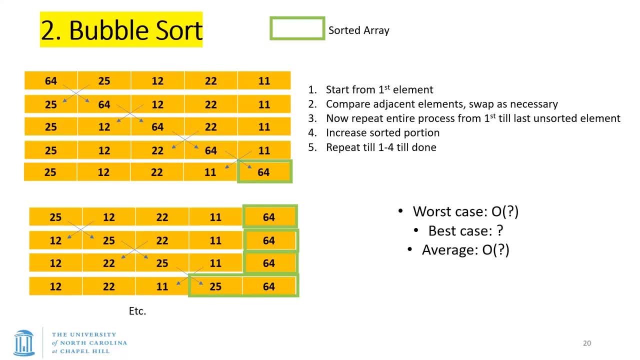 look at adjacent elements and if they're not in the right order, we'll swap them, and then we'll continue going on all the way till the end, and then we'll come back and do the whole process again and again, and again, until we've done it enough times. okay? so here's. 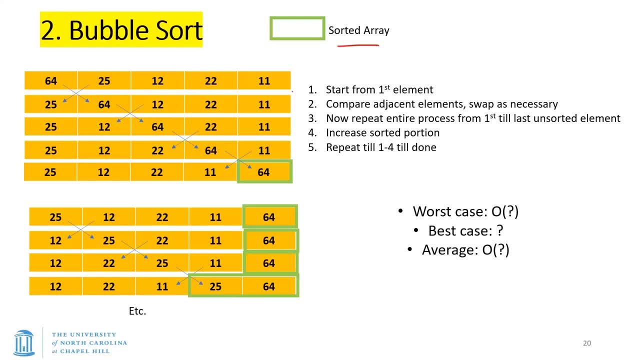 this algorithm again. it has a sorted component and an unsorted, so the green box is shown as the sorted component. We start from the first element over here and we compare adjacent elements and we swap as necessary. okay, So we compare 64 with 25.. 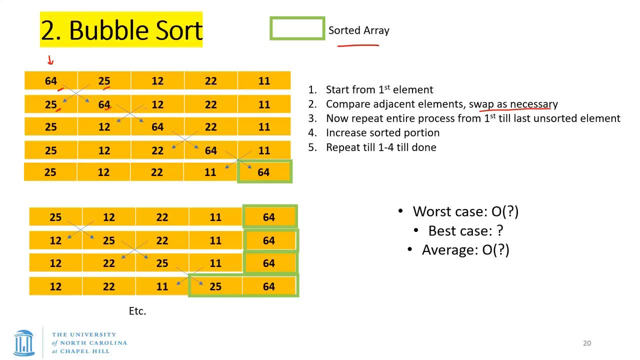 Well, 25 clearly is smaller, so we swap it with 64. Then we go forward. okay, We compare 64 with 12. So 12 is clearly smaller, so 64 goes up. So you can sort of see that the largest element. 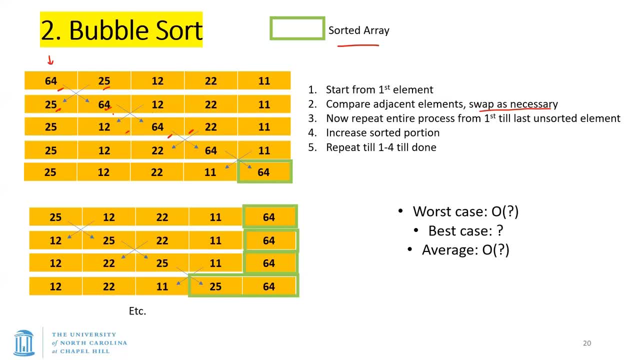 is sort of being picked to go all the way to the right. Okay, The largest element, which is 64, is sort of slowly being moved all the way to the right And as soon as you end up with the last comparison, the largest element has been selected. 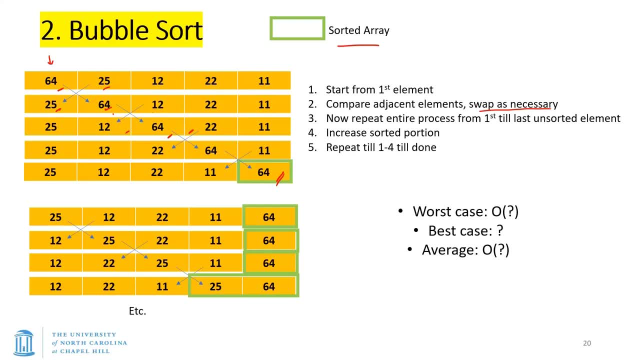 and is on the rightmost slot. And then we're going to repeat the whole process again, But this time we may not have to go all the way to the end. All right, So we're going to again compare 25 and 12.. 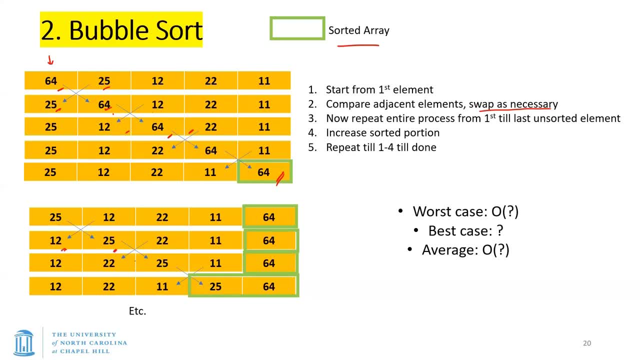 12 comes up here. Now we sort of pick the second largest number, 25.. As you can see, 25 is slowly drifting to the right, but we don't necessarily need to go all the way to the last spot. Why? 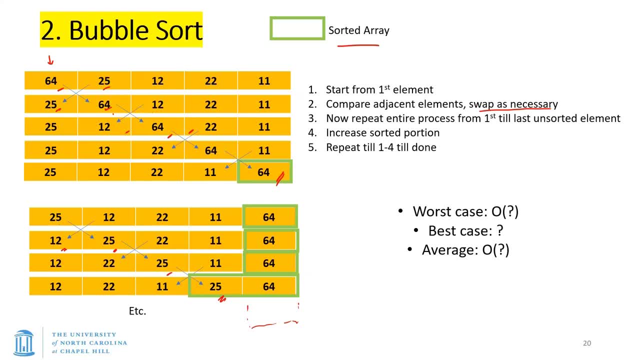 Because now we only need to go to the unsorted portion And every time we're doing one iteration, the sorted portion increments. Okay, So we're increasing the sorted portion and we're repeating all of these steps until we're done. So what is the worst case? complexity in this case. 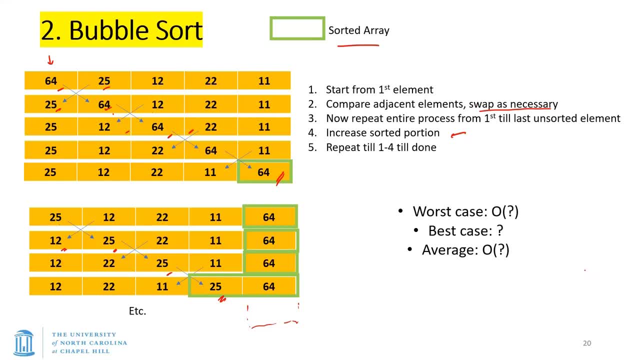 What's the number of steps? The first time around, It's basically n or n minus one. We go in comparisons, All right. So as you go down this entire series of steps, this entire series of steps is basically n equations, Right. 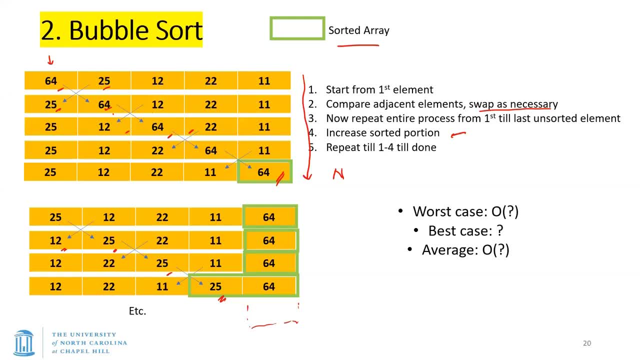 You're comparing um, you have n elements and maybe comparing them n minus one, but roughly n, or n minus one, but the second time around we go through one less equation, so this becomes n minus one steps and you can see again where this is going. so it will be. 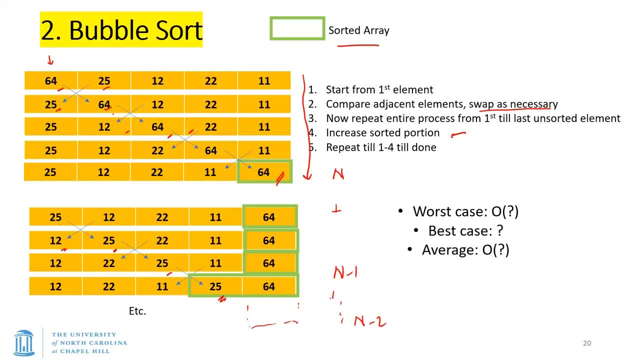 simply again, a sum of n plus n minus one plus n minus two, all the way until the entire, the entire array is sorted. okay, so that gives us the same result, which is order of n squared. so average. you can just take my word, for it is also. 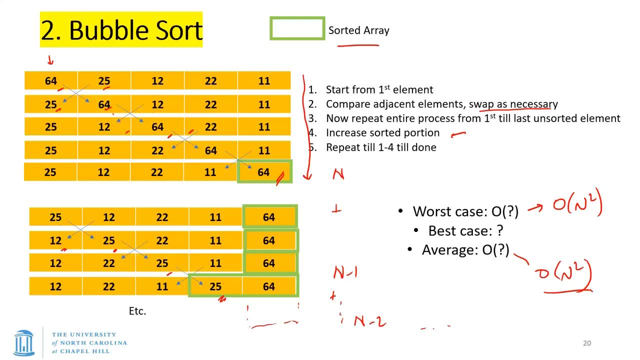 going to be order of n squared for a typical distribution, you know, randomly distributed. let's not talk about that. what about the best case? imagine that all of these numbers are already sorted: one, two, three, four. so now is it still going to be order of n squared? 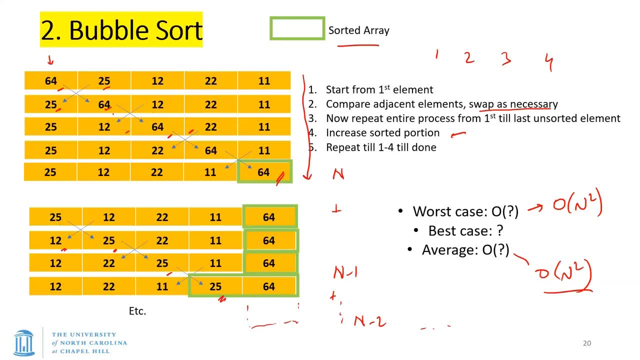 or can you make a almost a trivial modification to the algorithm and convert that into a better complexity and what could be that trivial modification to the algorithm? so we start off. we say, well is one and two, we compare these two, or one and two, and no swaps required. yeah, 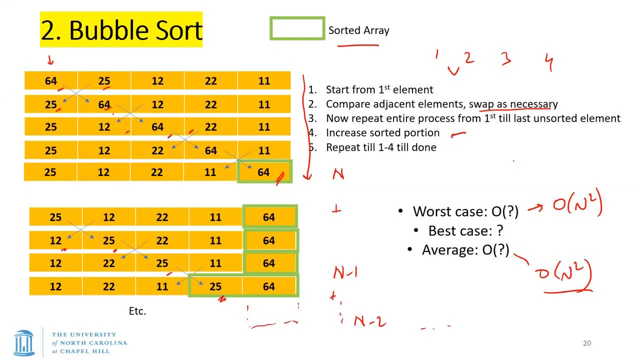 exactly so. if you are, if you're going through this in the first iteration, if you don't find any swaps- and that would be easy, that would be essentially part of the algorithm- all right. you're simply doing a swap and you have another flag, which is true or false- and says: was a swap done or not? okay, so if at the end, 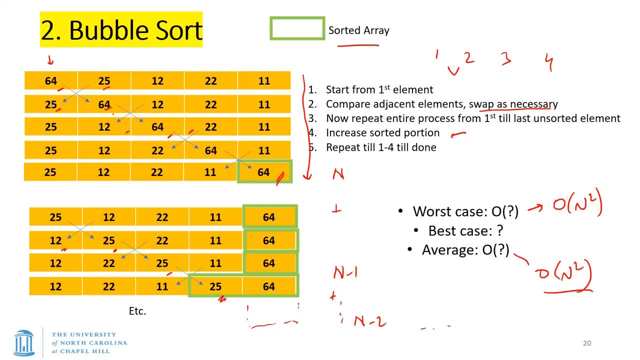 of the entire iteration we didn't do a single swap, then obviously that implies that the entire data is already sorted, so that's almost like a trivial modification and that would result, in the best case, which would be considered as order of n. okay, yeah, you didn't swap on the one category that you choose to say, that that one and two. 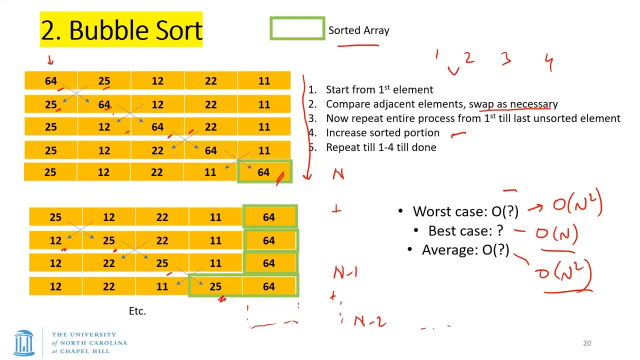 would be one item and you say: all four of these is the last item. that's right the same, as you know. all right, let's say it's like four, two, three, five, seven. so four, two, three, and what was the example? again five, seven. okay, so some. 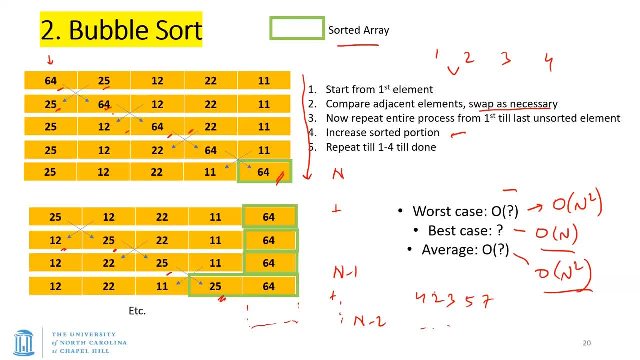 portion of it is sorted. two, three, five, seven are almost sorted. four is out of place, right. so can you come up with a different algorithm, or are you saying that, within bubble sort, can we sort of make a small modification and come up with a better complexity? yeah, you could do that. yeah, okay, so let's take a look. 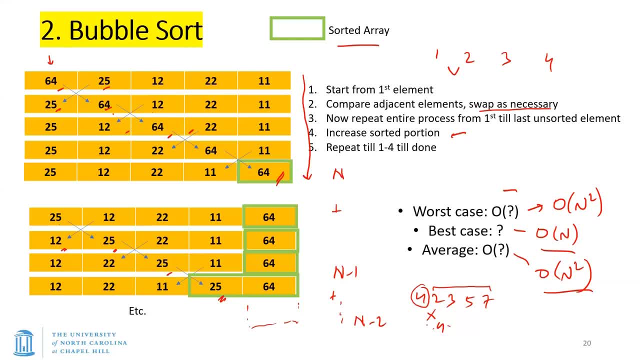 at this particular example. so four would come up here and two go there. all right, then you compare four and three and you're going to realize that three goes here and four comes up here. when you look at five and seven and you say no changes, no changes and essentially in one iteration. 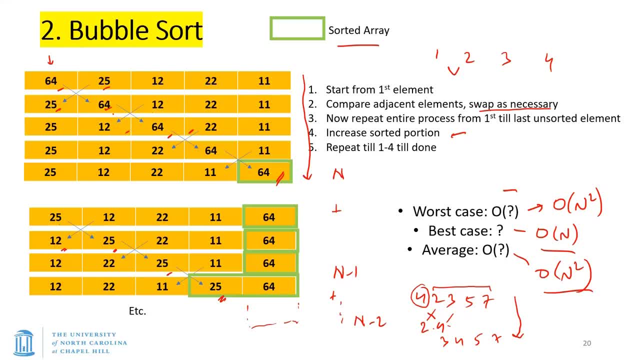 you have completed the job right, but but do we know that? do we know for sure that that is the right complex, that we've got a sorted list? we can see it as humans, right, but in terms of the algorithm, can you see whether is there some criteria that you can use? 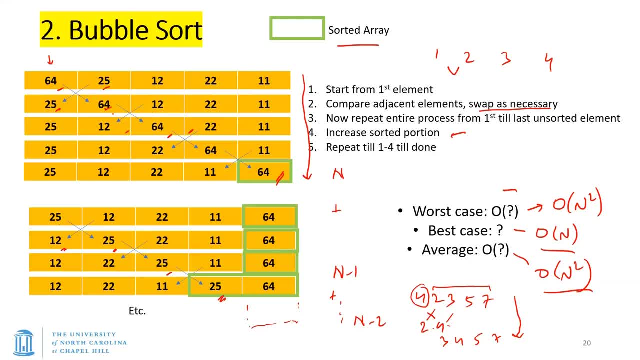 that would say that we don't need to equate any further. so you've got a great idea, okay, and that sort of relates to what the average scenario is going to be. okay, so, on average, some portions of this array are going to be sorted, some portions are not, and the question is, if it's, if this is. 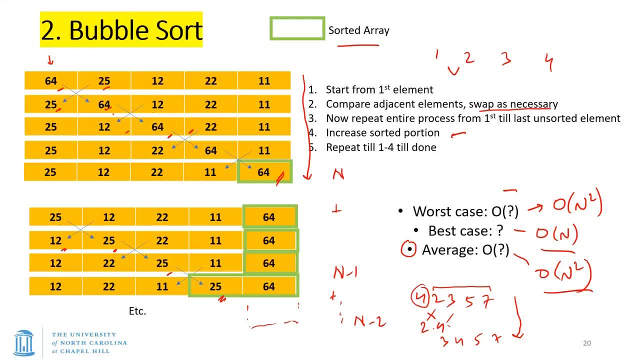 randomly sorted and some portion is. you know, 50 of it is sorted, 50 is not. what do you do? the average complexity: okay, so that's a more complex analysis, but it can be shown that on average is still going to be order of n squared. okay, but that's, that's the right. 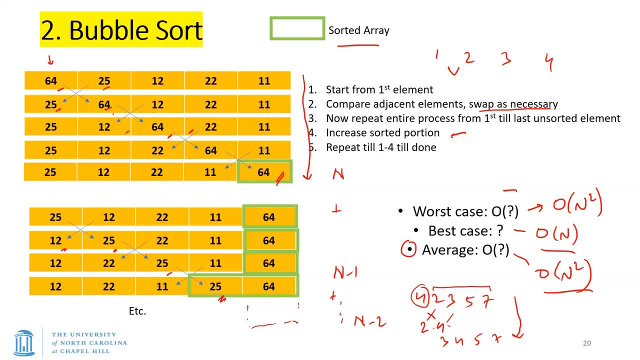 way to think about it. okay, and that way you can actually come up with your own algorithms, because you're trying to see, well, uh, in what scenarios can you actually improve the algorithm? okay, and that's great. so, um, so, unfortunately, in this case also the the average uh is is 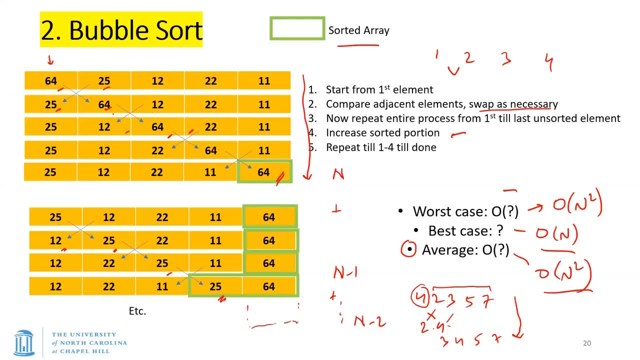 n squared, but the best case has improved right. so the best case, with a very trivial modification, is now superior. so now we started with selection sort. uh, bubble sort seems to be superior. but what about space? is it in place or not? is it using additional space, which is a function of n? now, so it's again in place. 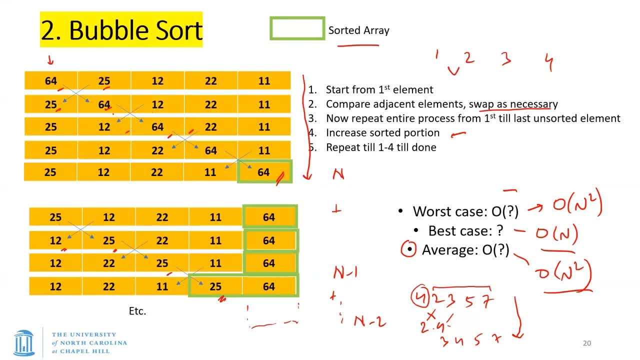 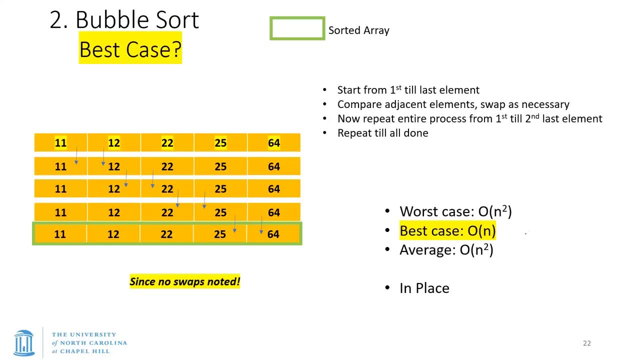 so it seems to be superior to selection. sort right, because, um, we've got the following scenarios and, uh, it's also in place, okay, so the best case has been improved, while the worst case- the average and the space requirement- is essentially as bad or as good as selection. 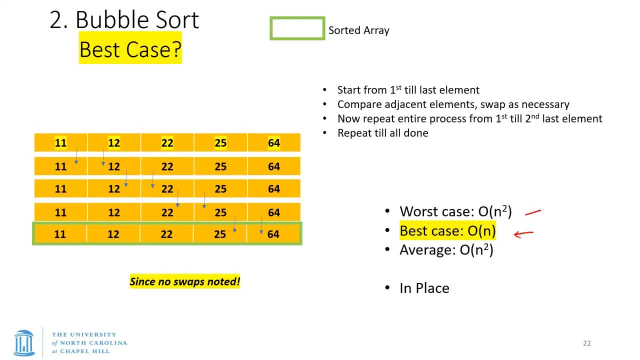 swap. so we're making improvements, okay. so these are two uh, fairly straightforward algorithms that you know. you don't even need to take a computer science algorithms course to be able to figure those out. you know, you could just think about them and it's kind of obvious. but now let's. 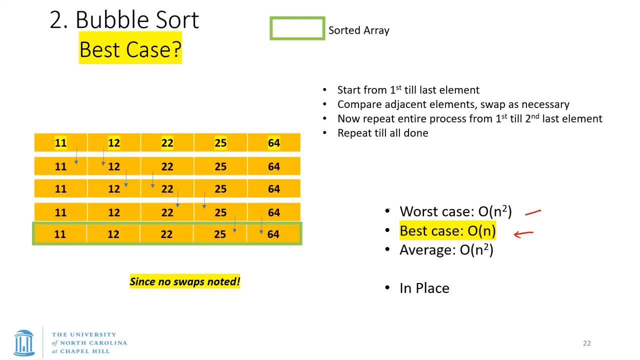 take a look at more advanced algorithms, where we basically look and try to see if the worst case phenomena can be improved in order of n squared, as you can imagine, is really bad right, uh, order of n was bad enough, but order of n squared is is far worse. okay, so now we're going to take a look at. 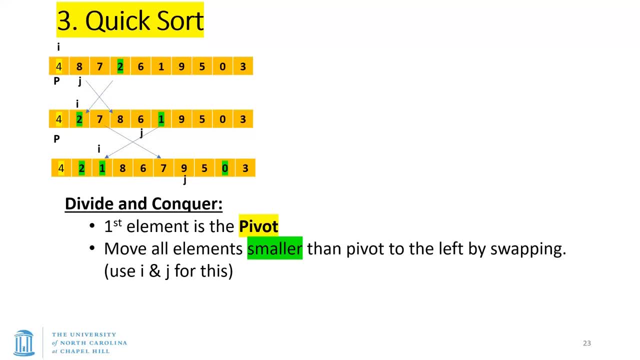 um, which is sort of a generically referred to as um, divide and sort sorry divide, divide and conquer algorithm. okay, so there are a whole bunch of algorithms which, uh, try to divide the problem into smaller portions and try to resolve the small problems. okay, um, can you think? 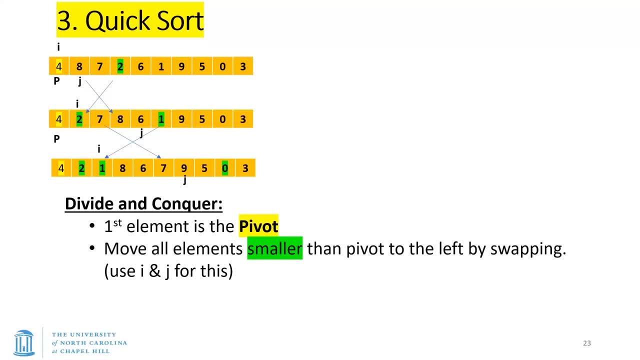 of any algorithm that we saw. again, going back to our first few lectures, which can be thought of as divide and conquer, yeah, recursion, okay. so basically what we're doing is we are, uh, whenever we're doing a recursion, we basically say: well, in order to solve this problem, what we can do is make it slightly smaller. 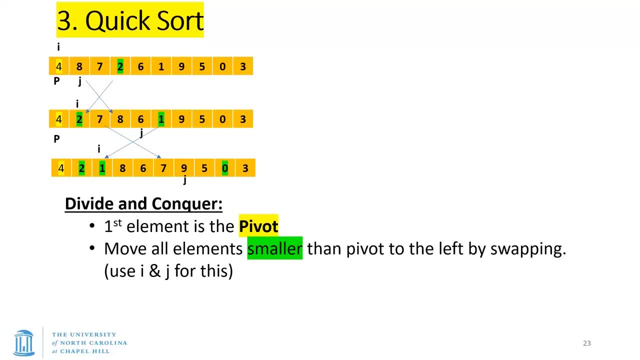 and keep on iterating until we actually rather recursing, until we get to the base case and then we move backwards. okay, so that's a great example of divide and conquer. okay, um, not saying what the complexity is of those scenarios, but let's think about an algorithm that we just thought of a little while earlier for doing a search in the second lecture. 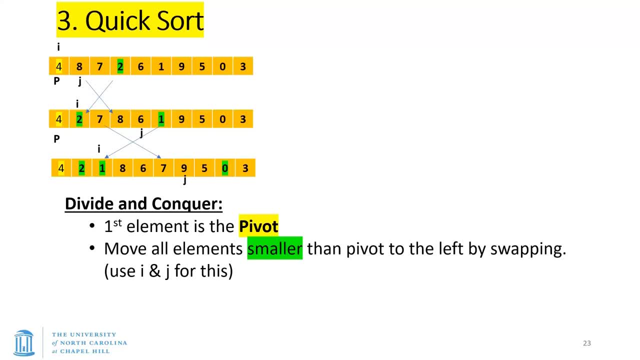 which was the binary search. okay, in binary search, what are we doing? we're saying that we're assuming that the data is sorted, but now, in order to be able to search through that, we say, well, let's start from the middle and we compare the number that we're trying to search for, whether it's smaller. 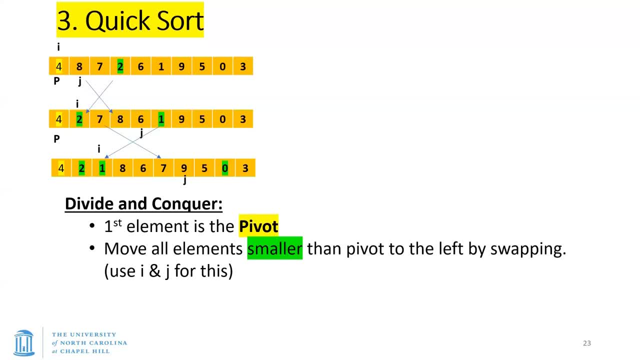 or bigger then the number that we found in the middle, and if it is either way, we divide up the search space into half the size and then we simply have to work on that particular half. and then again we go to the middle of that portion and we say, well, is it to the left? 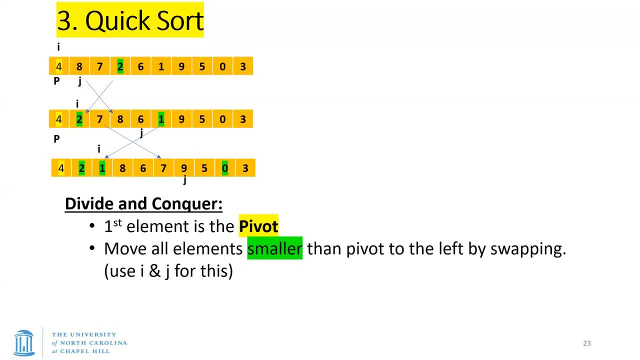 or the right, and then we divide the search space into half again. so every time we are going through a binary search, we're dividing up the search space into smaller and smaller portions. so it's sort of like dividing it up and then conquering that particular part. okay, so that's sort of a general way of thinking. 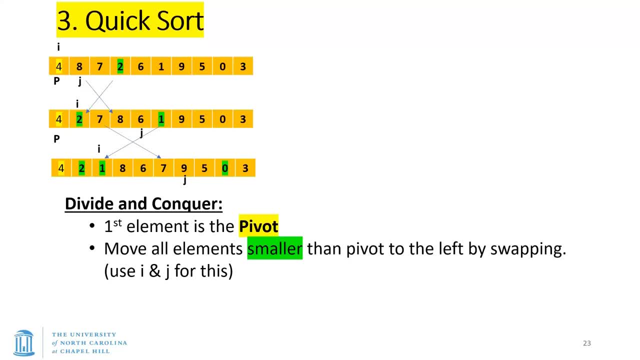 about it, and so quicksort is sort of similar in that sense. okay, it's going to divide up the space into smaller portions and then try to resolve those smaller portions separately. so let's take a look at this particular algorithm, which is referred to as quicksort. it's a little bit. 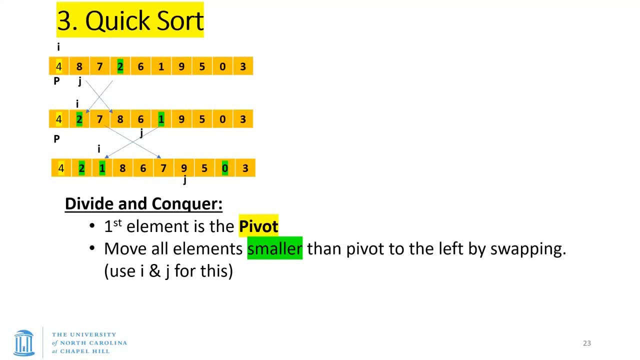 complex, but hopefully in the next few minutes you should be able to get your hand in around it. so what it's going to do is it's going to use the first element of the array and we're going to call that the pivot. okay, so starts off, takes the first element and it calls it the pivot. i've 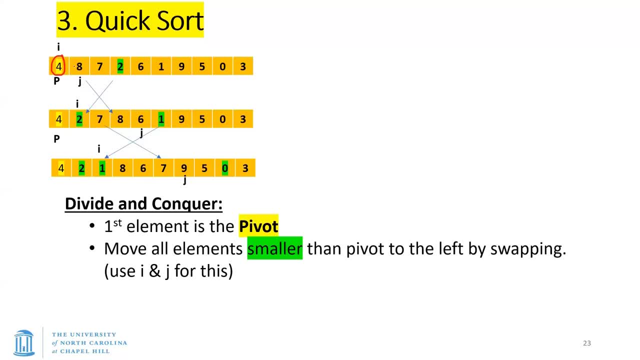 shown that as a yellow, it's shaded as yellow, and then it it goes through the rest of the array and and it compares these values with the pivot, and every time you come across an element which is smaller than the pivot, you swap it. okay, swap it with what? let me show you so. 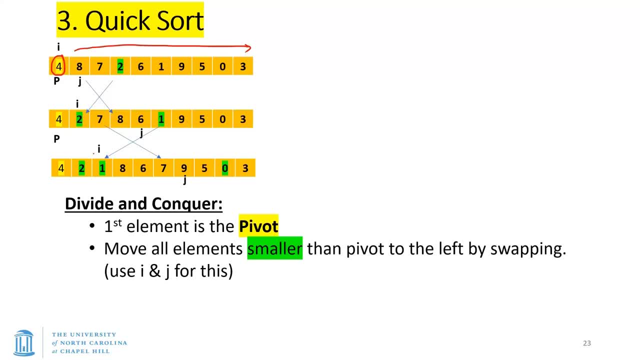 i is. the location is one location, which is where the pivot is. and well, let's just forget about i and j. let me explain this to you in general. you go through the first element, the second element, you look at eight and you say, well, uh, eight is not smaller than four. 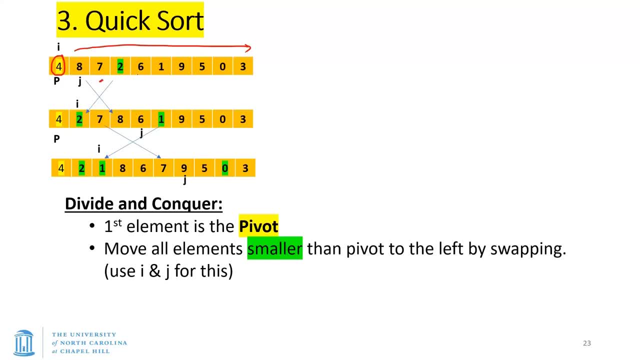 you disregard this. you go to the next element. seven is not smaller than four. then you go to the next one. you find two is smaller than four. okay, so we're going to swap two with eight. all right, so the element which is next to the pivot- so eight- goes in two's location. 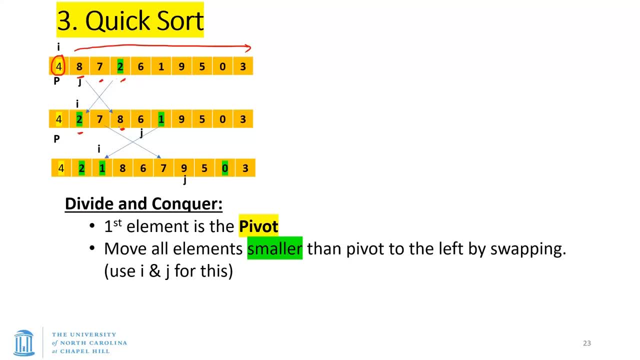 and two goes in h location. all right, we continue on from that point onwards. so we continue on from this point onwards. we say, well, is six now smaller than four? no one smaller than four. yes, so now we're going to swap it with the next location, okay. 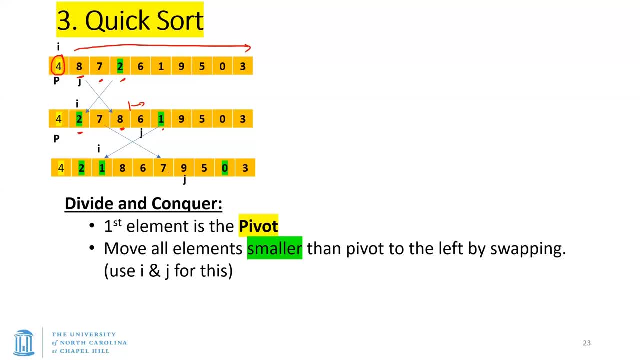 so one goes in the location of seven. seven is, uh, moved up to one spot. we continue going onwards from this particular location. nine is not smaller than four. five is not smaller than four. zero is smaller than four, so we're going to swap zero with the next location, eight. 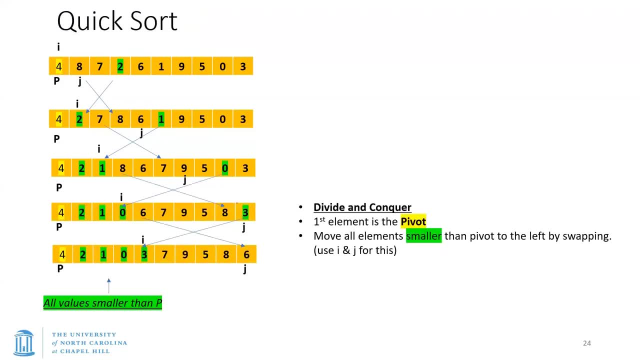 okay. so if you look at the next slide, we swap zero over here, um, and then we continue on. from this point onwards. is three smaller? yes, three is also smaller than four. so now what you see is that all of the values which are smaller than four are now all the way on. 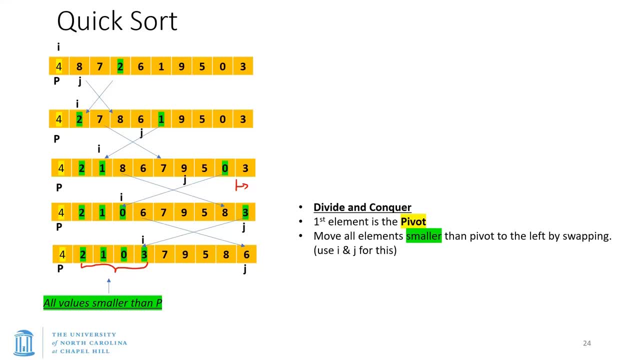 the left side. all the elements which are bigger and we're assuming distinct values- all the elements which are bigger than four are to the right side. okay, but are these elements sorted themselves now? so all the green elements internally are not sorted. it's simply saying that they're sorted with. 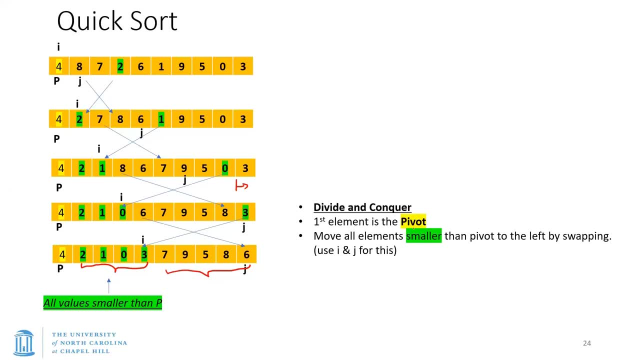 with respect to the pivot. okay, um, so that's what we've initially done. the next stage is that we want the pivot to be in the center. okay, another way of thinking- this is an example that i'd like to give- is that, uh, imagine there are a bunch of kids in school. 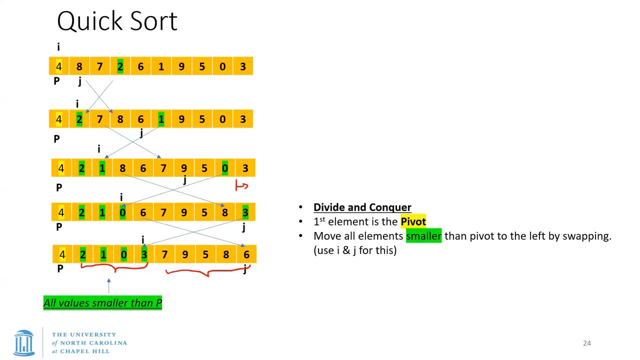 and the teachers just ask them to get sorted in the order of height. okay, you want the left, the shortest kid on the left, the tallest kid on the right, okay, so now, one possible way that the kids could do this is that each person looks on the left and the right and says, well, um, perhaps 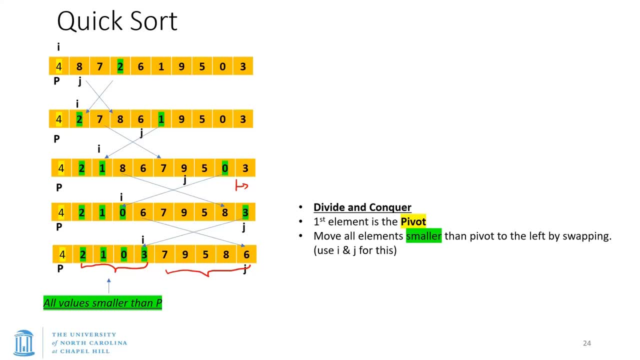 about average in height. so i'll sort of go to the center of the room, okay. and then the rest of the kids say, well, okay, am i taller than this kid? uh, if they are taller then they go to the right of that kid, the shorter kids kids go to the left of that kid, okay. so you can think of this initial. 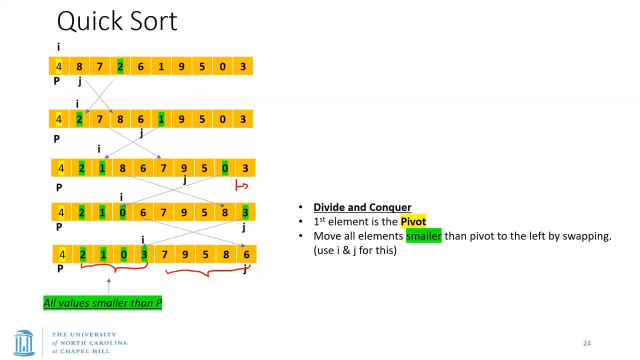 chap as a pivot. so what he or she has done is he's anchored himself, they've anchored themselves in the middle and all the kids which are taller and now on the right, all the kids which are shorter on the left. the kid with this chap is now in the right location and he's anchored himself in the 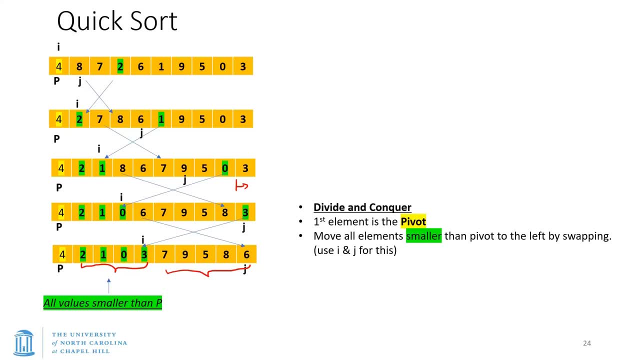 left location and he's anchored himself in the left location. can you see that? okay, so this person doesn't need to move any further. now the question is: how do we get the pivot to be in the right location? so we've done the initial portion. now we just need to make sure that we get the pivot to be in the right location. 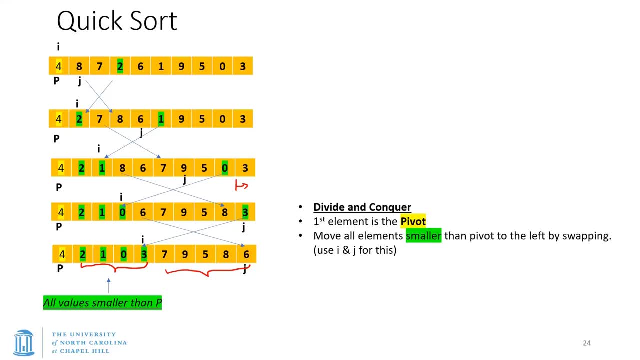 so how could we get the pivot into the right location so that the pivot doesn't have to be swap? swap it with the middle, okay. so what we could do is we could take four and swap it with three. okay, so three comes all the way here and four comes here, so does everybody. 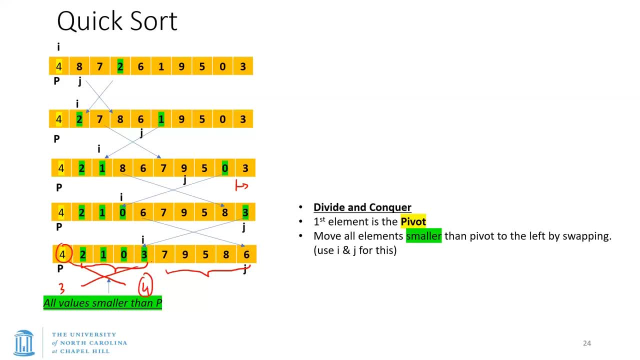 see that, and once we swapped it with this chap over here- this three, then four- the pivot is now in its perfect location because all the elements to the right are bigger. all the elements to the left are smaller. okay, uh, is that the best way of of getting the pivot? 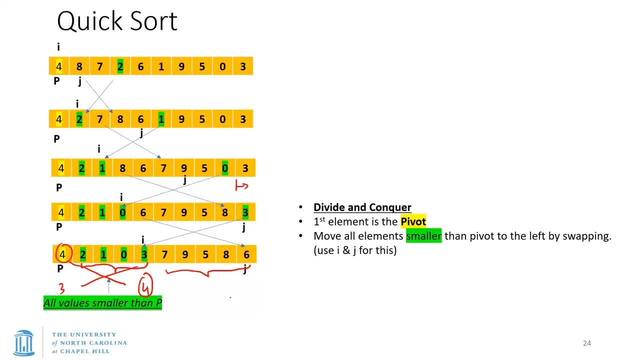 to the middle. would there be another way? what if i suggested that let's move each one of these guys by one, so that four, four goes in three space, but two, one and zero are shifted, each on the left and then one on the right, and then one on the right and then one on 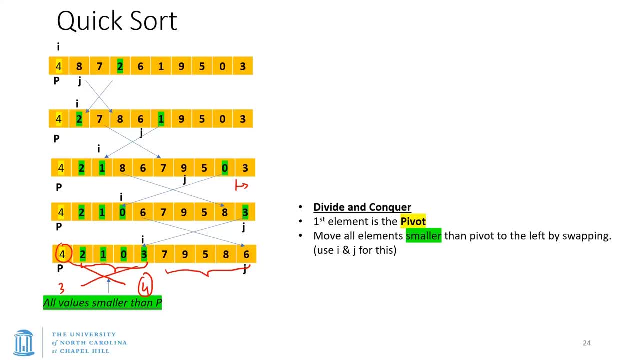 them are shifted by one. does that make sense or that would that be worse? so let's say i said: well, we could have two, one zero being shifted, and then we have, sorry, two, one, zero, three and then four, which is the pivot goes over here and the rest of the elements going here. is that superior, or what you suggested earlier? 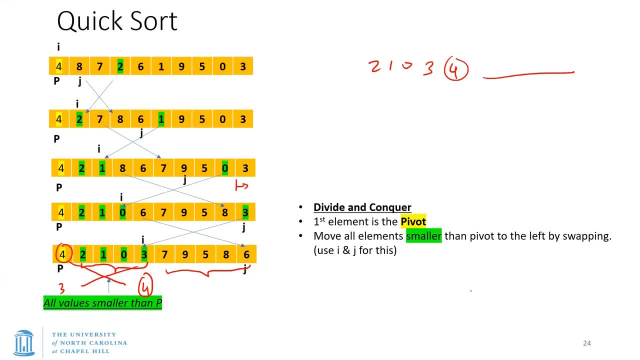 is simply to swap four over three. yeah, one, two, three and then three and then five, exactly, exactly. so i want you guys to think about that now, because, just to make sure that you guys are awake, so obviously, uh, swapping makes more sense. okay, if you didn't swap and 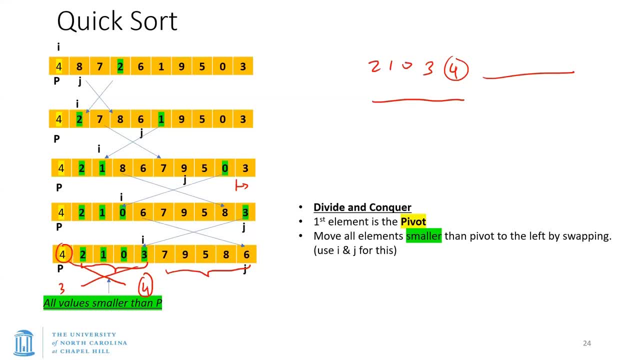 you shifted, then there was no point in shifting them, simply because they're unsorted, all right. so there, there doesn't need to be any special relationship between two, one, two, one zero and three. okay, so now we have the pivot in the right location. now we can just move on. to the next one, so three. so now we have the pivot in the right location, and then we have that pivot, and then we have the pivot, and then we have the pivot. okay, so that gives you that pivot, and then we have the pivot. so if we want to move on to the next one, here, let's 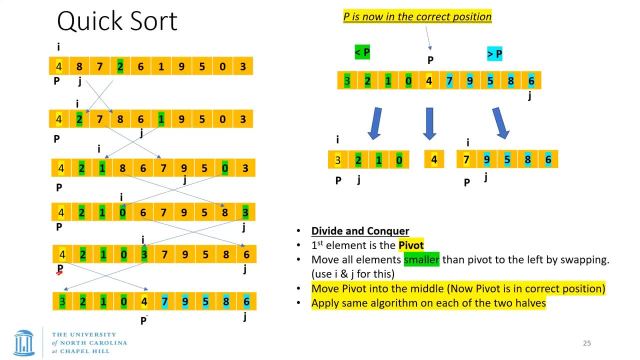 location. we've swapped pivot with this middle cap and we have three over here. uh, and then two, one zero, are in the original location. four is now in the center, roughly in the center, and the rest of the elements on the right are bigger than the pivot. okay, so that's the first iteration. 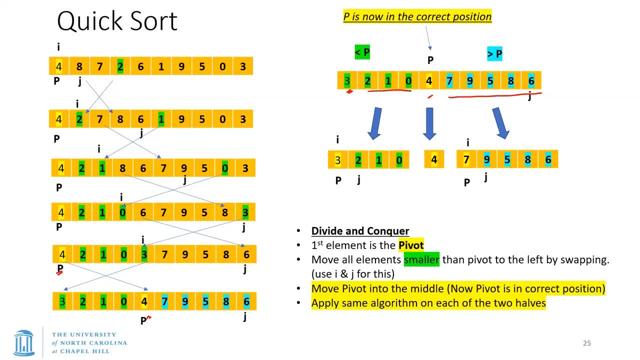 how long would that take? what's the complexity of the first equation? we've started with the leftmost, we've selected this as the pivot and we've simply said: well, we're going to go down and we're going to do some swaps. so what's the complexity? 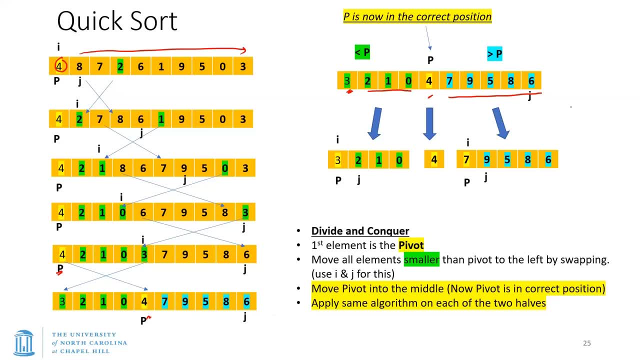 we go up, yeah, so all the way down, uh, to get to this stage, it's simply big of n? all. right now, the question is: what have we achieved? well, remember, this is uh, divide and conquer, yeah, uh, yes, yeah, we've got good, uh intuition over there, and but we need to figure that out, okay. so, um, 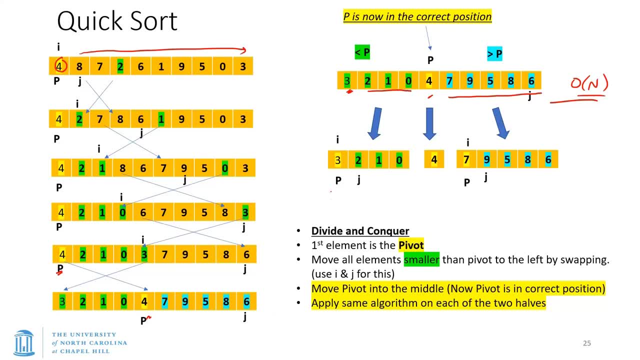 so now what we're going to do is, you can imagine, is now we're going to use divide and conquer. okay, so now we've divided up this problem into two smaller operations. the left portion four is in the right location. the pivot is in the right location. the left portion is in the right location. 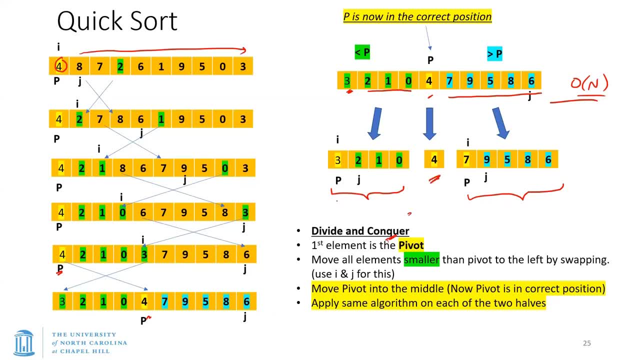 and now we need to sort the left half on the right half, so sort of similar to a binary search. okay, sort of similar. however, how is it different from a binary search? if you think about, at this stage, in binary search, we also divided up into a small portion, into a left and right, and here we also 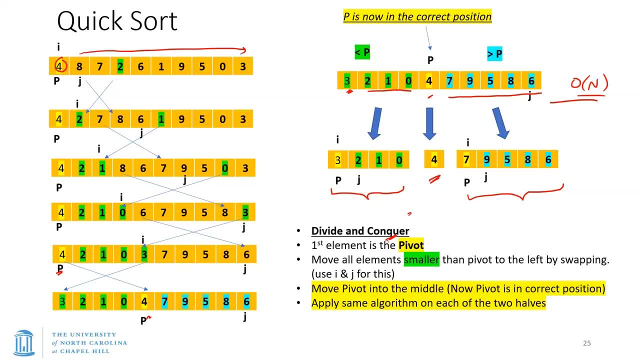 dividing up into two parts, smaller, and yeah, sorry, can you speak up a little bit? yeah, exactly. so in binary search we said, well, we're looking for an element and now it's either in the bottom half of the top half right, and so now we have to disregard one half and we've reduced our search space. aha, 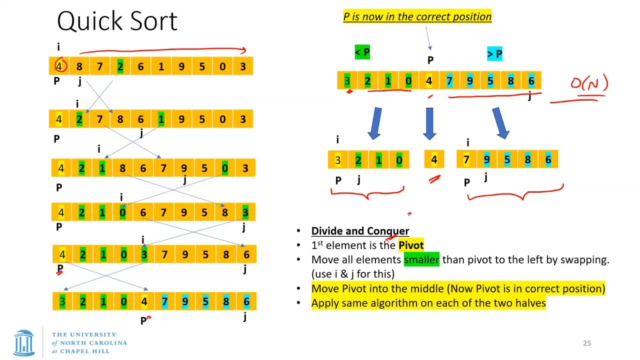 in this case. can you do that? no, we need to sort the entire thing, unfortunately. okay, so now we need to sort the left portion as well as the right portion, so the complexity is different from a binary search. okay, that's why the gentleman over here mentioned that it's going to be n log n, but 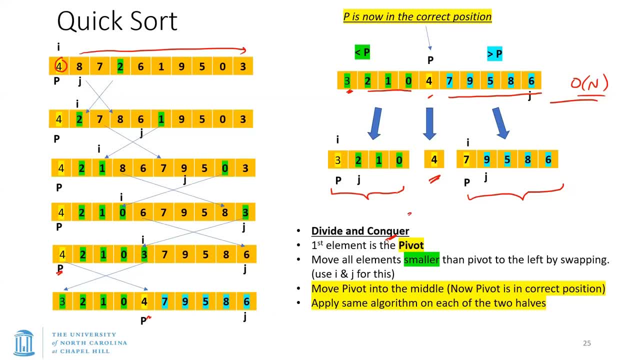 let's figure that out, as opposed to a binary search, which is, which is what? just log in. okay, but here you can already see there is a difference and you- uh, 550, you actually figure this out why it's mathematically, why it's different. but here we sort. 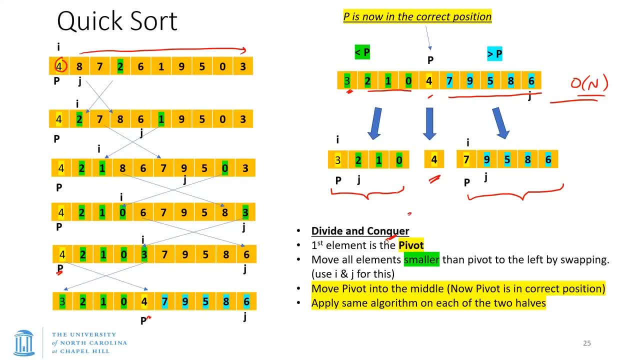 of do it in a simpler way. well, so let's take a look at now what the complexity of this is going to be. so the first operation was m steps. what is the complexity of the second step now? we have two halves. each one of them need to be. we're going to recursively apply the same algorithm. so now, 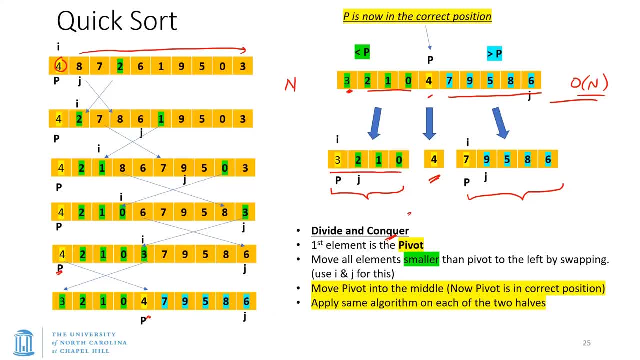 we're going to say, well, this is the entire array, so to speak, and so we're going to select three as the initial pivot. for the left half, we're going to apply the same algorithm, and for the second half, we're going to use seven as a pivot and we're going to use the same algorithm. 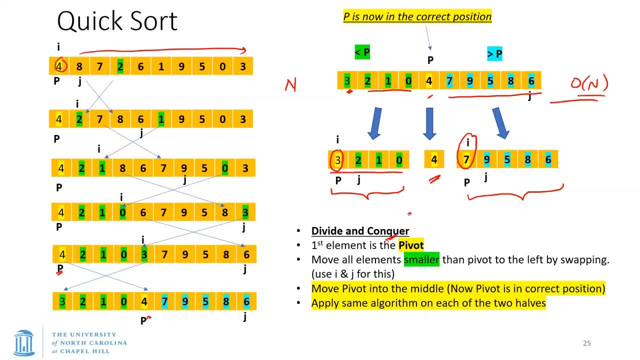 okay, so now what's the complexity of the second phase? so this one can be thought of as the order of n. yeah, so is it half of n? this is half of n, right, and then this is also half of n, so it's not just half of n. 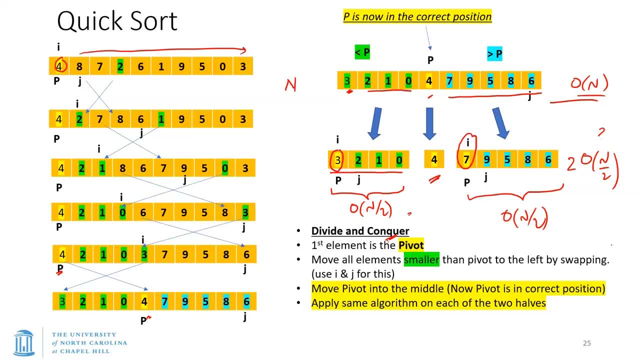 it's two times half of one, all right, so two times all different upon two. that basically becomes that it's essentially n okay just doing this half, which is that part two. the other half, which is n upon two, and those two added together are essentially n disregarding the pivot okay. 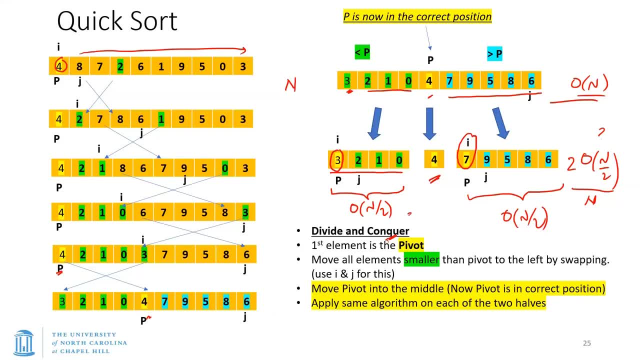 um, so it doesn't seem like we've achieved much. okay, we just divide it up into a more complex situation and we're still doing n operations. okay, now what happens as you go forward? what about the next stage? so this is. this can be thought of as two times add upon two. 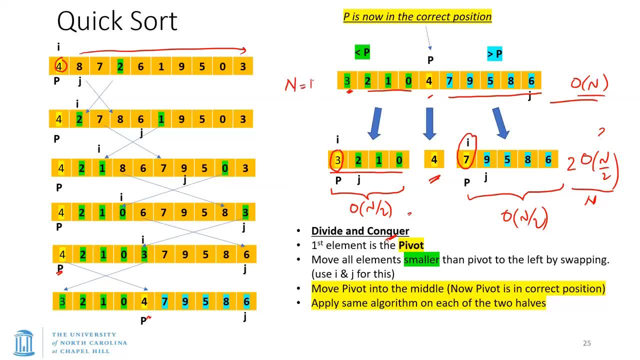 now imagine that n was 16.. now we've divided up into two times 16 upon two right, so 2 times 8.. this is also 16.. in the next stage, what's going to happen? we're going to divide it up into smaller portions. all right, so this is going to become smaller and 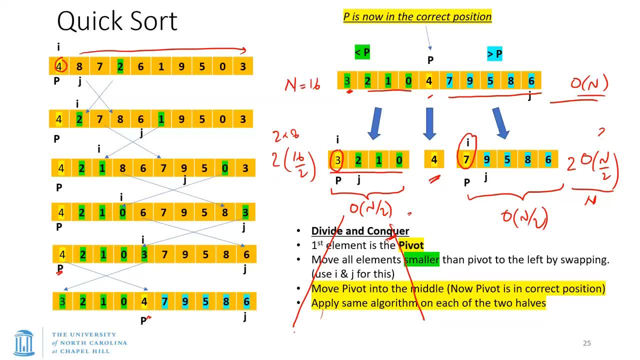 so on, so on eight. we're going to have eight points. so let's say: this becomes eight, this becomes eight, so this becomes become four and four. this is going to be four and four, so it's going to be four times four. right again 16. so what's the point of all of this? yeah, 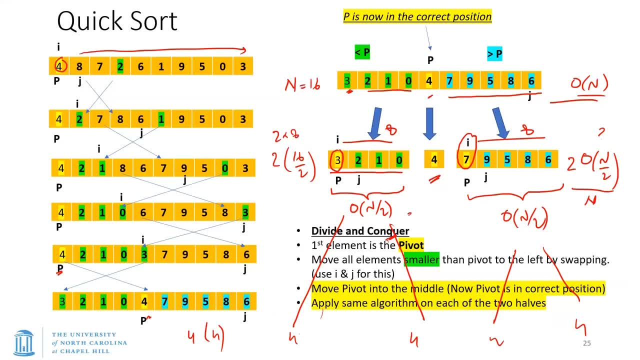 exactly so, ultimately, this number over here is going to be equal to one, for in the next stage is going to be eight times two. the next time it's going to be 16 times one. okay, so each one of those iterations is going to take 16 steps, but so what was the point? 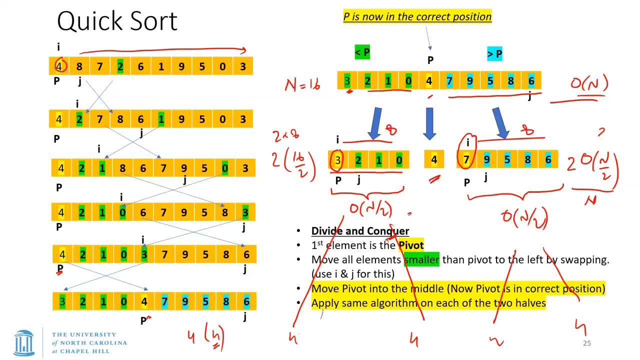 what is the point? yeah, how did you get n log n? that's my question. we're looking at the the worst case, so it's not looking at the best case. we had the right intuition, but we need to figure out how we're getting or in log n. 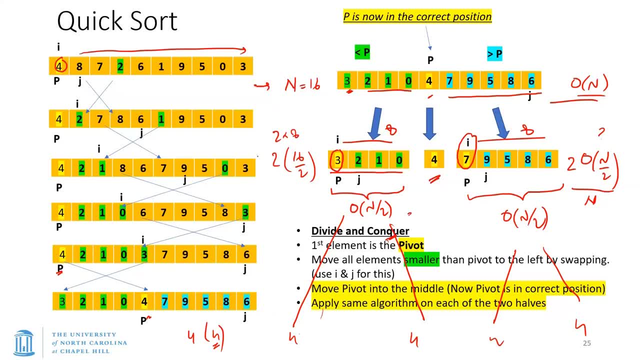 so we have n steps, okay, then n steps again and then n steps again. but how many times do we have to take n steps? what do we need to multiply n by by? are we doing n iterations, or are we going to be doing fewer equations? what somebody? how many occasions are we going to be doing so? each time you're dividing it up by half? 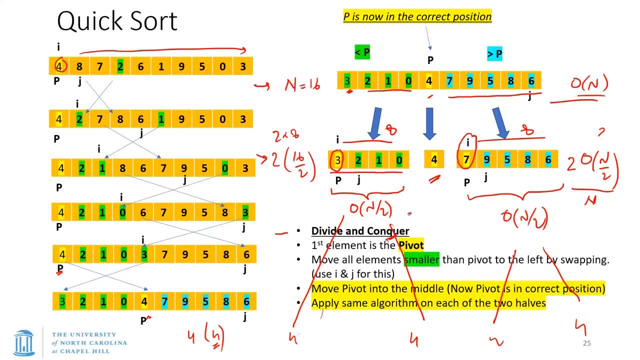 right. so 16 becomes eight, and then it becomes four, and then it becomes two and then one. so how many times we have to do so? how many times did we have to repeat the entire process? five times, right times, right, and so five. we do it socially, right. yeah, take an 밥 after you take a break, right? how many times did we have to repeat the entire process? 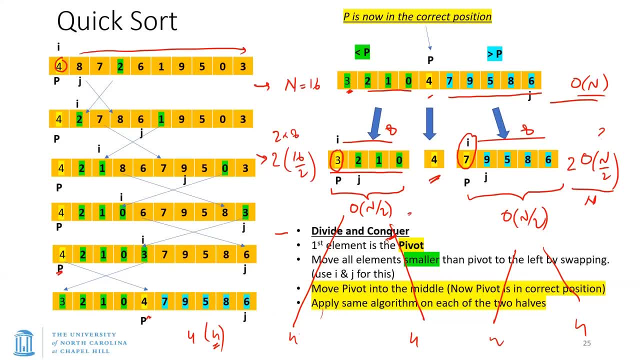 five times right, and so five. we take n steps again, right. so how much i st soccer, and then you take that extra step right, um? so, because these iterations, you know, are all p is 질문it B, a in some scientists. you know how to do them, okay. so if you do, they don'tribe. so how many times did you have to repeat the entire process? five times right, and so five times right. online you have t p. he'll stay. hey, tips talking strategy. huh, this is a crazy thing, hi, i didn't get rid of it.